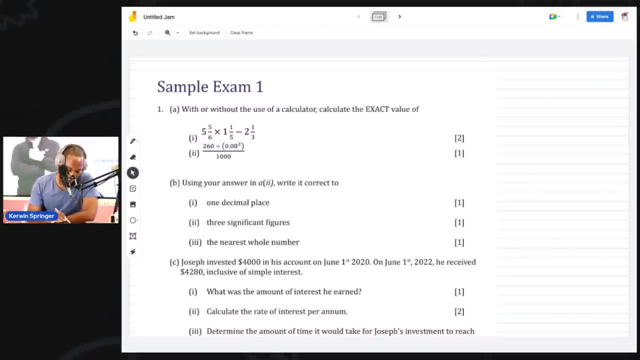 I'm using Google Jamboard. Well, not first time, First time in a while. Normally use another one. So they want you to do the exact value So and they say with or without the use of a calculator. So I could just straight up put this into a calculator and get the answer. That is the. 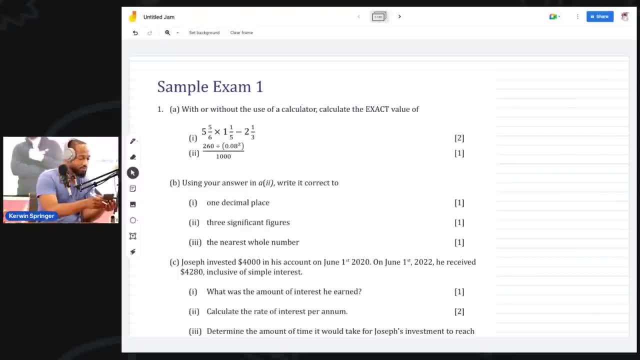 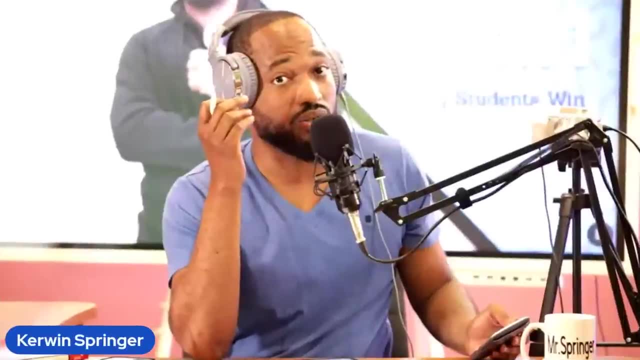 very first thing I want you to do in the exam. So, like you, actually the first thing you do in the Maths exam is look at question nine, the circle geometry question, And you think up of all the ideas that you have to find the angles and you write it down as fast as 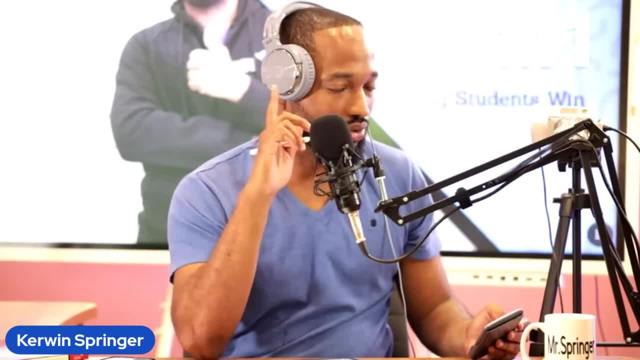 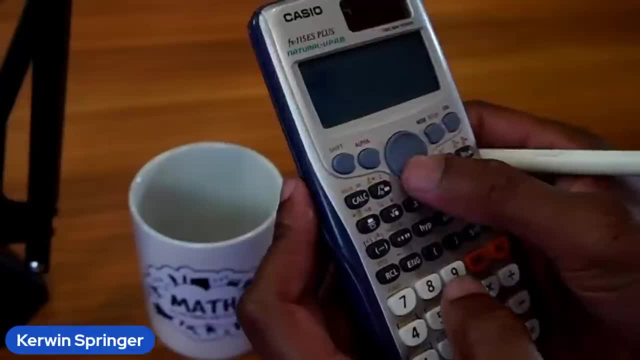 possible. And then you go back and do question one. So, but when you start question one, I have to say: use a calculator, use a calculator. I have to say, use a calculator, use a calculator. just make sure i get the answer and you'll see my calculator there. you see how i love, why i love. 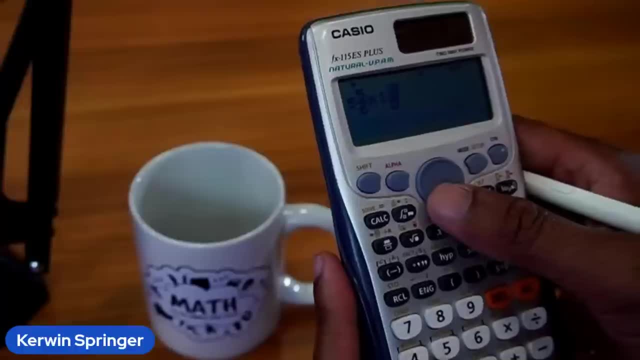 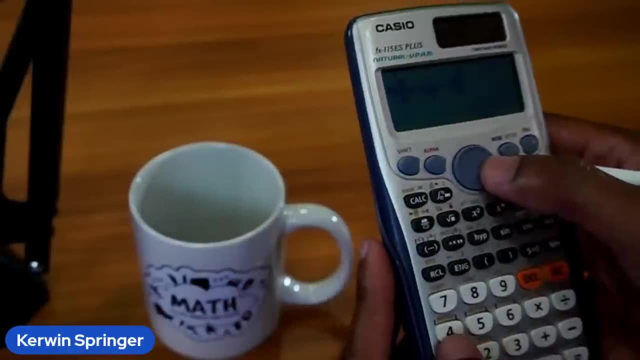 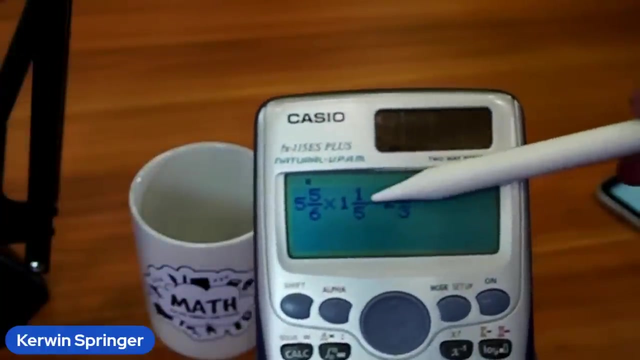 this calculator you can just put in the fractions, naturally nice and proper, and this calculator will organize bud mask for you, everything. so you can literally type the answers. you see it on your paper. type it just so you see it on your paper and press equal boom and we know we're looking. 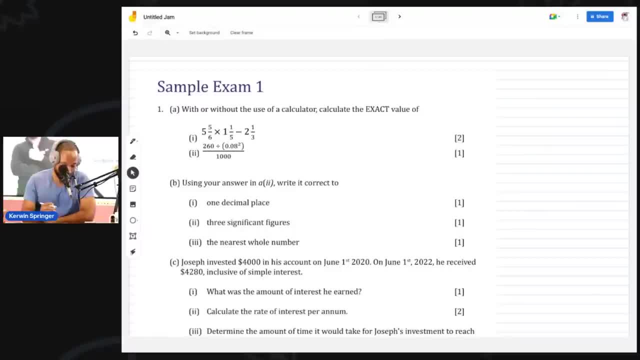 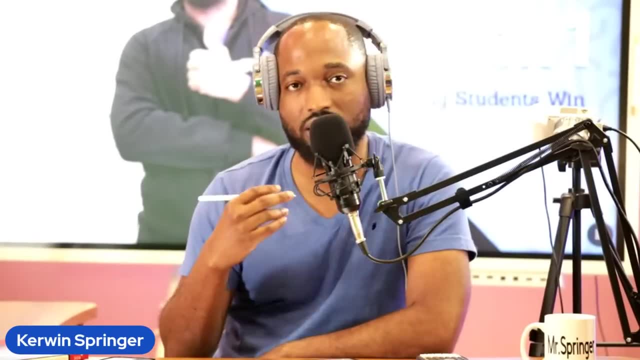 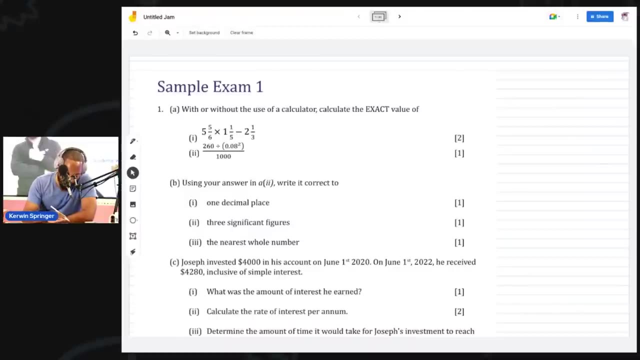 for 14, over 3, of course. um, then, after you do that, i would advise that you write it down and you do the lcm stuff. if you had to do lcm stuff, you multiply it out. i'm going to show you exactly what i mean. let's see if i can reach through this. um, where's my pain? let's make it blue, how about? 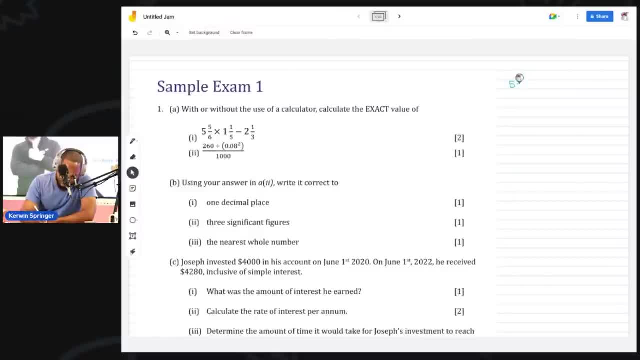 blue. so let's say five and five, six multiply by one and one, fifth minus two and a third. you'll see not properly on the screen: hello samantha. hello gamer alex. hello chicken curry, boy chicken curry. i don't need to ask where you from. five by six is 30 plus 35 over six. multiply by one by five plus six. 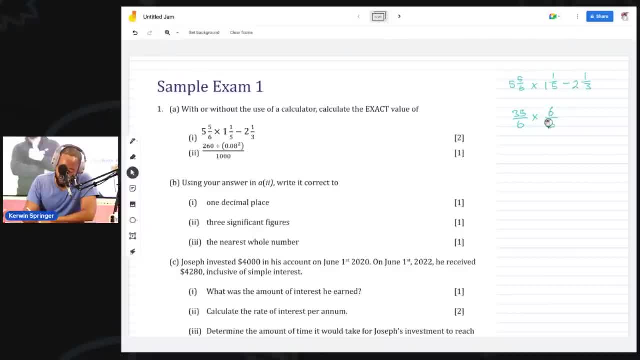 plus one is six. hopefully you know what i'm doing here. if you don't know what i'm doing here, you're in a rough place, my friend. two by three plus one, seven over three. i just want to congratulate all the golden state warriors fans. you know we need to do this separately though, so that part here separately. cancel this. 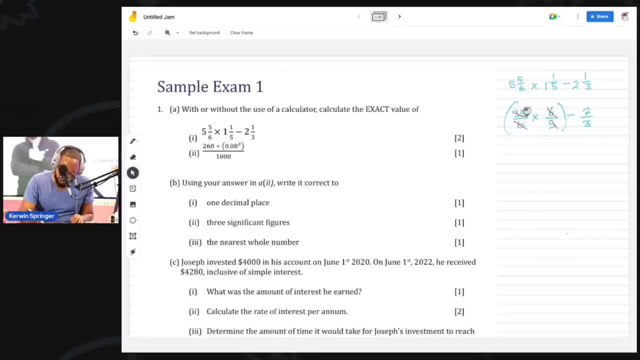 six and five can go into this seven times. so wait, what you're really telling me here? this is really just seven minus seven over three. now when you have a whole number like seven and you see in the denominator here, this is going to come in the exam for sure. so if you don't know this fraction, 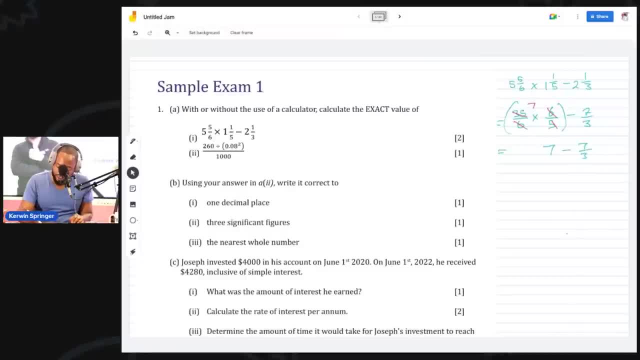 trick. learn it. what you need to do is say that this number seven is really something over three. so so we can have the common denominator, isn't it? but what over three gives me back seven. so it's literally: you're just taking three and multiplying it by seven and you're going to get 21. you knew. 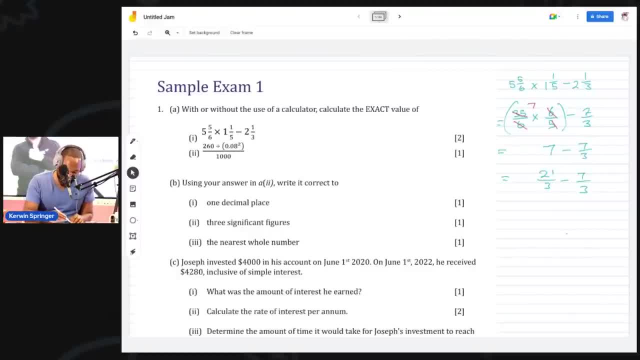 that you know that trick by joseph way. um. so so we end up now with 21 minus seven, which is 14 over three, and you have your weekend and you also have your answer from your calculator here that you can back it up. so we show, we guarantee that we get two marks in the exam already. um, the 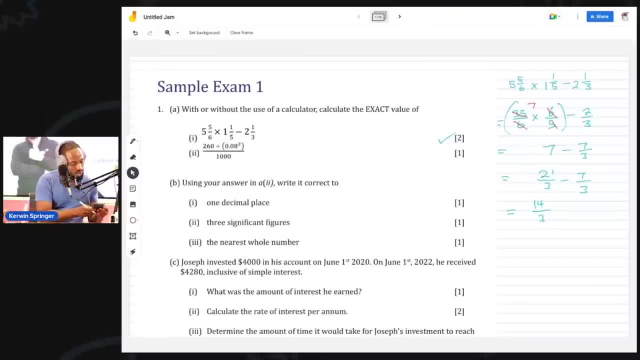 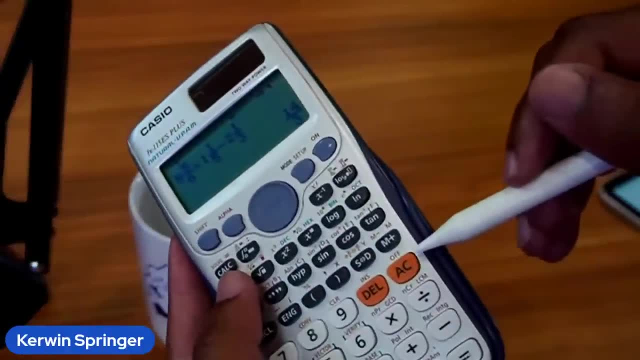 next question is the same calculator stuff. so what i'll do is i'll start off with a fraction. now, i don't like to press this button on my calculator. that clears off everything. instead, press the ac button. i give you only tips right through this. right, you're getting tips, right. 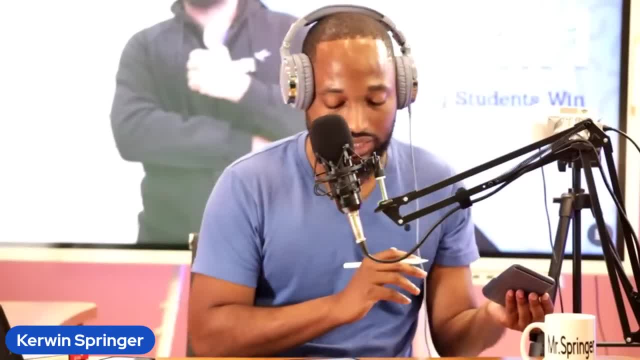 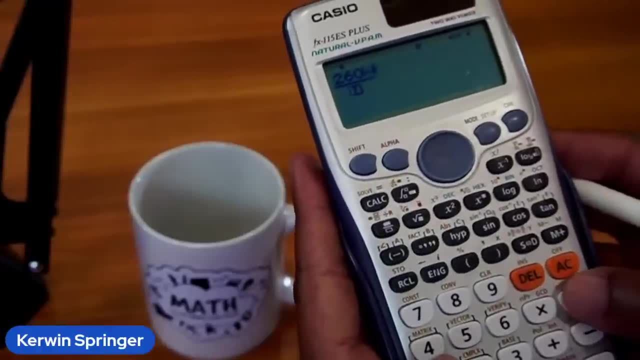 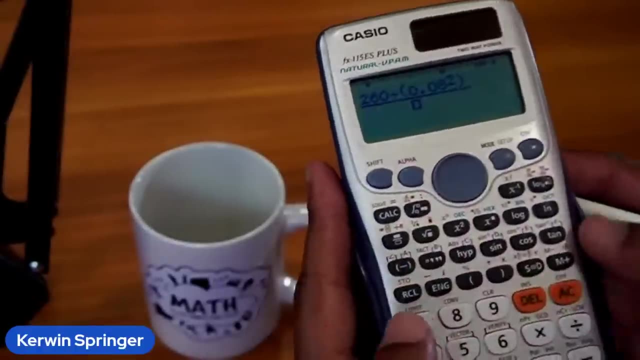 through this. so pay attention again and just bring up max in your exam. so you press in this one and then you're going to put 260 divided by 0.08, to be squared every day, every weekday, for the next two weeks. in the middle of the day you will catch me. 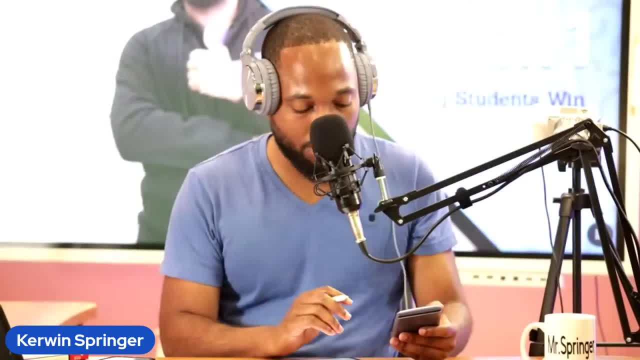 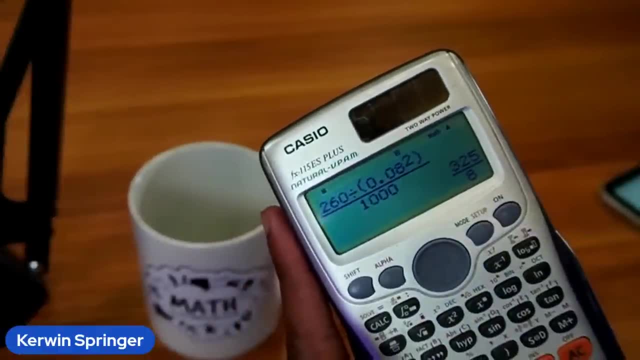 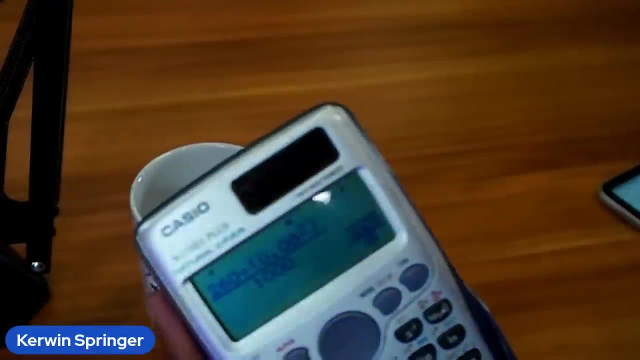 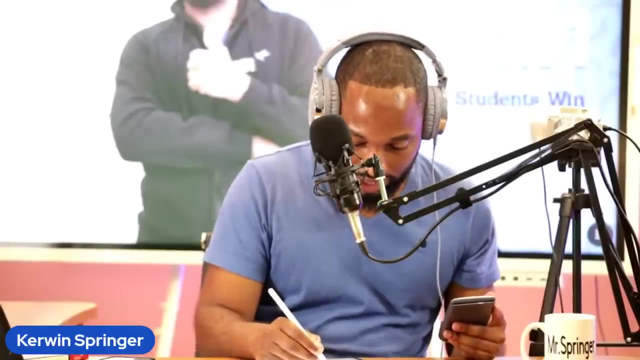 here. so what we see in my- i kind of pull it out of the screen- it's. i got this: three, two, five, eight, over a thousand. um, this one is just straight up calculator. now anybody in the chat can tell me why i am not going to, i'm not gonna, i'm not gonna find no decimal awareness here. why would i just leave this as an? 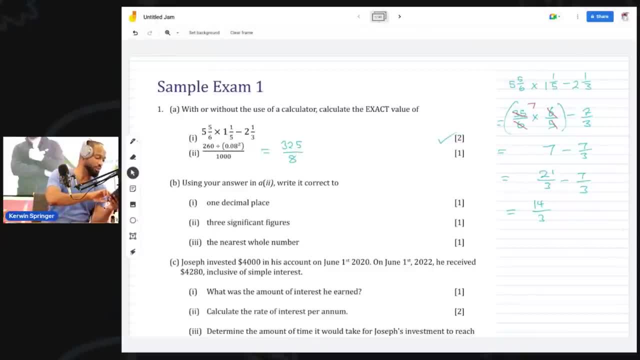 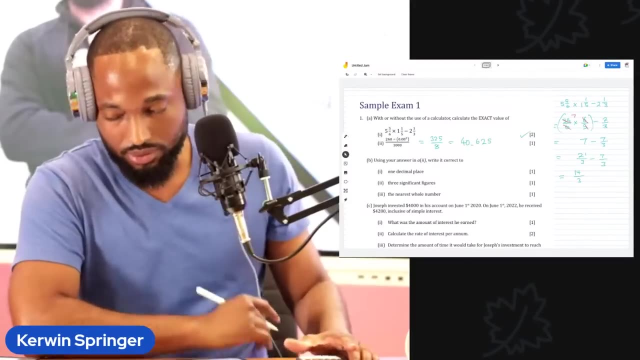 improper fraction and be confident now to switch the decimals. i can press this. i can also put 40 points, 40.625 in a class point, a character point. in this way, 0.625, I could also put 40.625, but what I definitely cannot do is put 40.6 and say approximate in. 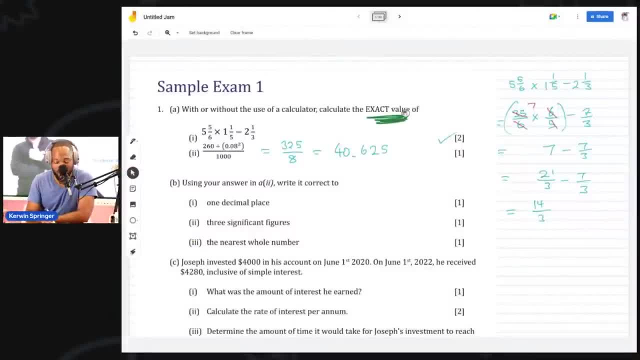 And the reason I can't do that is because they want the exact value. So, exact value, you would either leave it as a fraction or, if you have a decimal, you need to write the full decimal. Now, if you see a decimal places going on, and on, and on and on, that's an indication that you can't figure out an exact value, right. 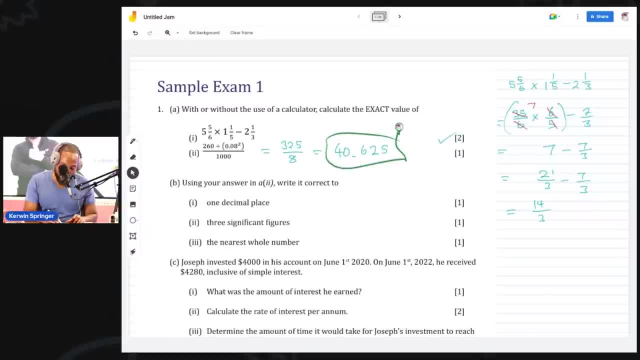 So this could work in this case, but I would advise that you just leave it as a fraction. anytime they say exact value and you collect your marks, right? Yeah, you're adjusting, you're correct, so you want the exact value. 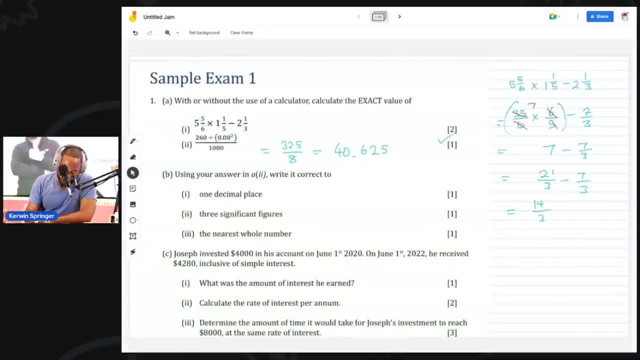 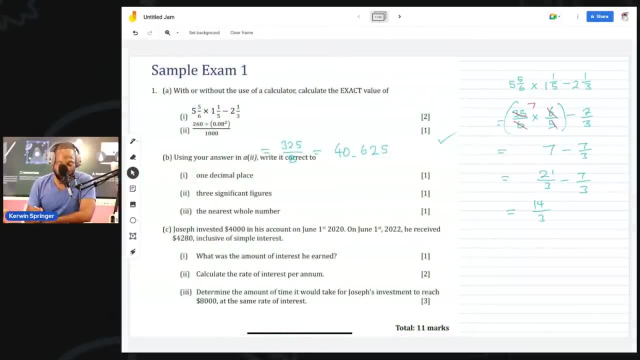 So let's go on. We're just doing question once a day. These sessions would be no set of trauma, no trauma involved. Let me just make this thing a little smaller again. a little too big for the boobs. Notice how this question is out of 11 marks. It usually is not out of 11 marks, right? 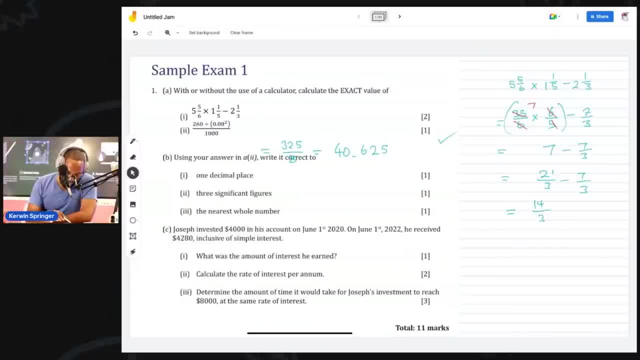 Using your answer in- let me just erase off this, Remember a little new- and now coming back in the game with this Jamboard Google Jamboard thing, Using your answer in E part to write it correct to one decimal place, So we know that it is actually 40.625. 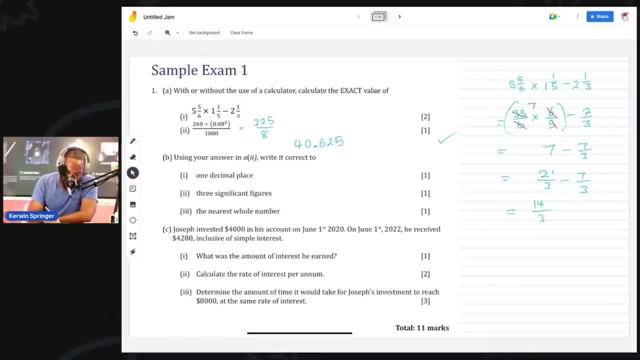 And if I want to get this to one decimal place, I would have to watch this decimal place here right And realize that what comes after that is a two. it's less than five. So what's it? to one decimal place, 40.6.. 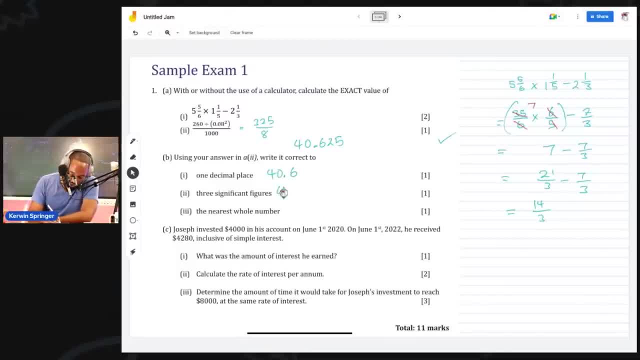 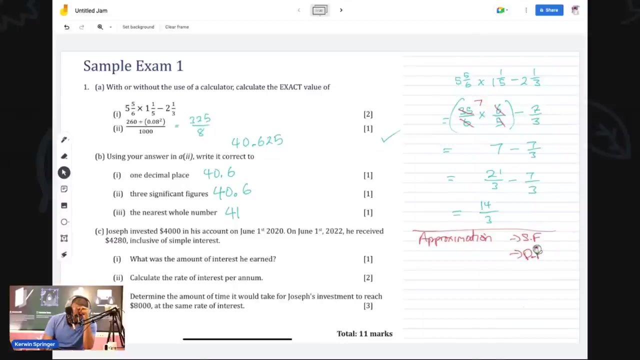 And the three significant figures, still 40.6.. And to the nearest whole number, 41.. Why is it in the chat if you understand that All of those who understand must know your approximation in the exams? Approximation in the exams, you must know. approximation to significant figures to decimal places, whole number, approximation, whole number. 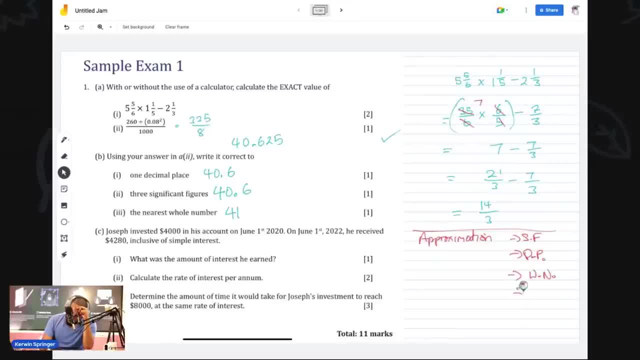 You could occasionally get some kind of place value approximation to like the nearest 100 or 10 or something that could come out in something. But that is normally SCA stuff. So they literally test you on all three in this here. So the next part of question one is consumer arithmetic. 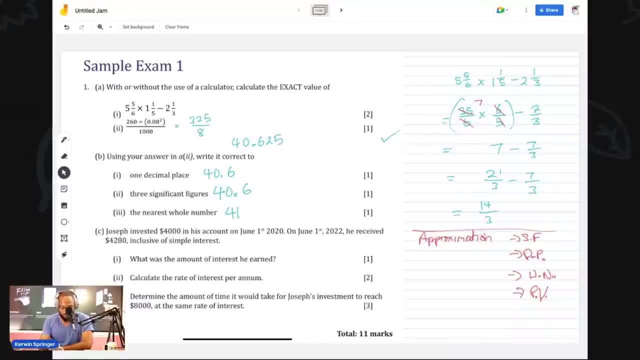 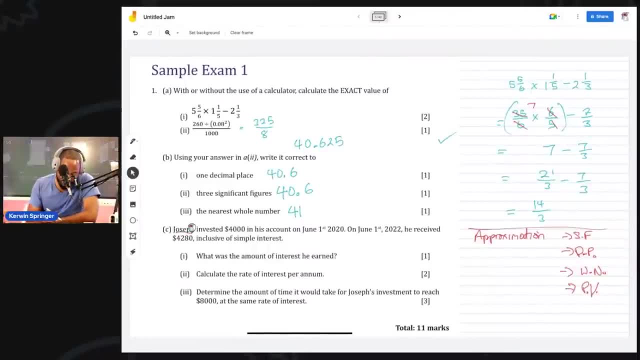 And let's see what they have in store for us. I might have to be switching between page one and page two, right, But I'm on page one right now, So stick with me. So, Joseph Invent. Joseph Invent invested 4,000 in his account on June, the 1st 2020.. 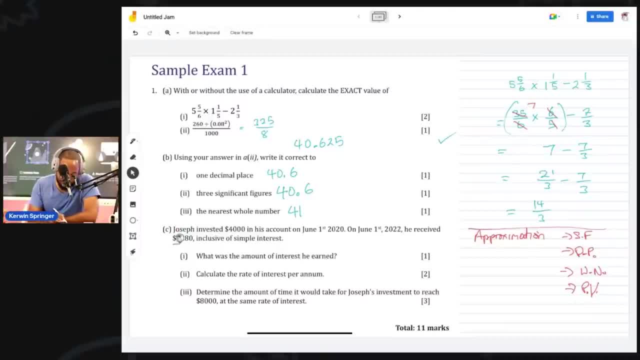 And June, the 1st 2022,. he received this amount in Exclusive of simple interest. So this is his full amount, his full principal, And we've seen the principal being included here, So he started off at 4,000.. 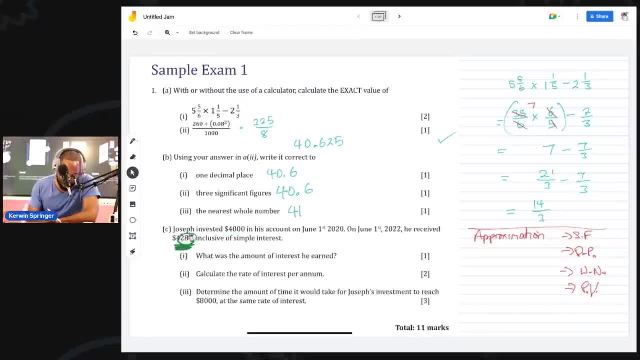 This is his principal: 4,000 plus $280 interest. So what is the amount of interest here? I done answered that already, So let me go on to page two and talk about that. So the interest- the formula for that is interest- is equal to the amount. 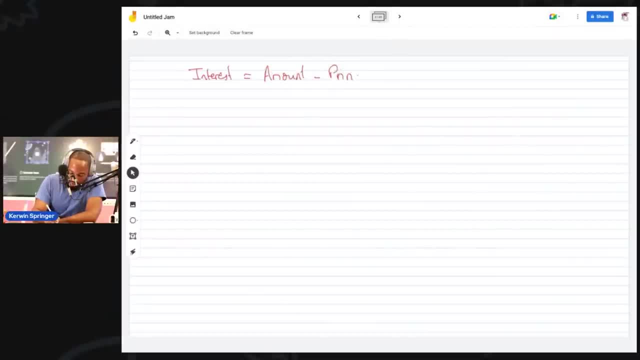 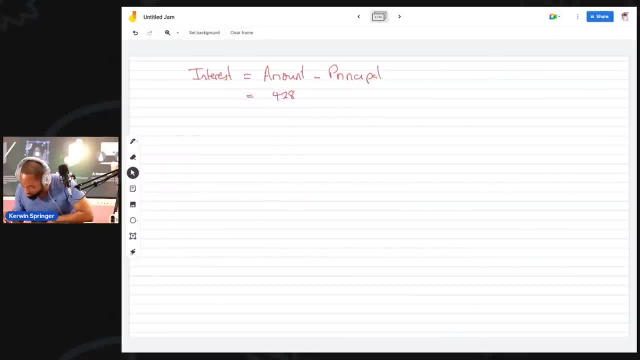 4,280.. My memory is undeniable Minus 4,000 was the principal. So the interest- and this is just for one mark- is 2,8.. Now you might be surprised, because a lot of students when they see a question with interest 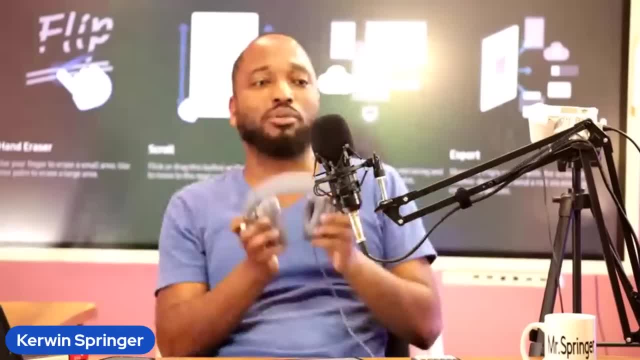 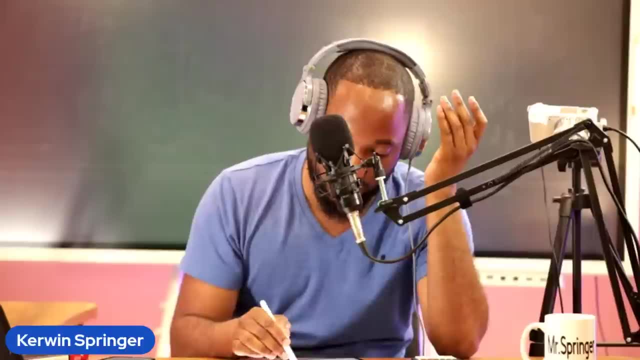 the only thing they want to hear is: mind to think of is simple: interest is principle, by rate, by time of 100, so they don't even think to just minus the amount minus the prince is like. is it's so quick to see, right, let's go back to. 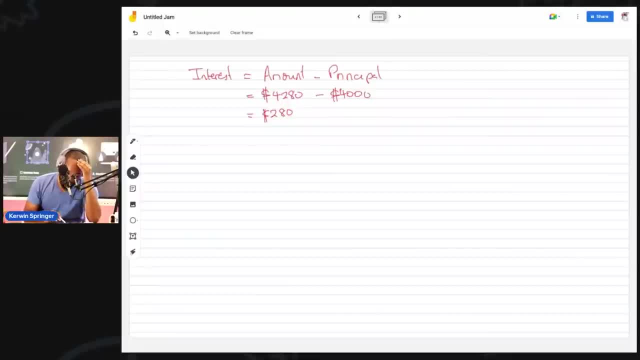 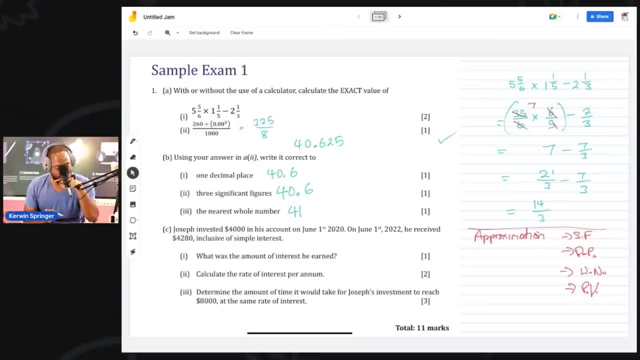 page one you can see that we have joseph investing 4 000 and at the end he received 4 280. so the interest is the lecture does he get. but every time some people hear about our interest, you're only thinking one formula, and don't be surprised. cx is going to ask you about interest and you're going. 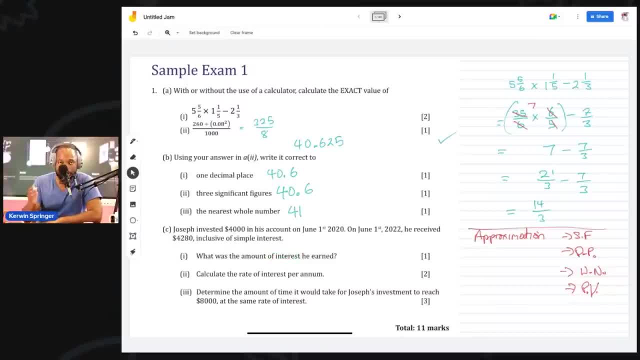 to just have to say the amount minus the principle. it's not always going to be simple. interest is principle by rate, by time of 100, remember that. so now we calculate in the rate um the rate of interest per annum. so the rate of interest per annum is kind of easy to see because it's 280. 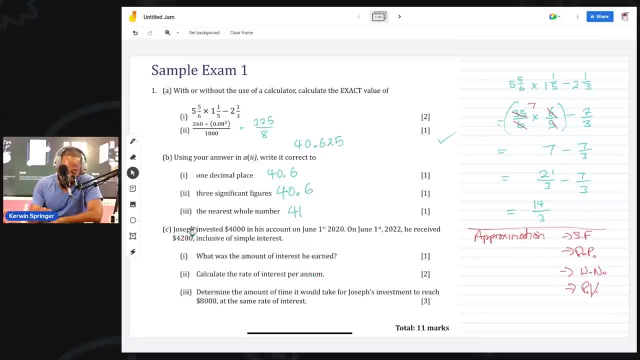 dollars. you divide it by two and then you put it as a percentage. but there's a formula that we have for that. who knows the formula for rate? so all of the formulas you have simple interest times 100 and then you divide by the other two things. 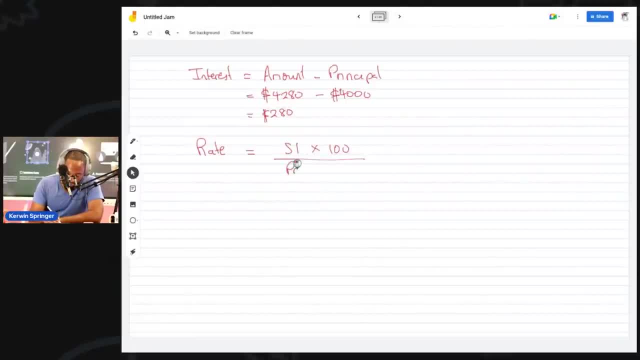 so in this case we're using rate, so it's going to be principle by time and just um for your information. like, if we want to work out principle, it's going to be simple: interest times 100 over rate by time. if you want to work out time, it's going to be simple: interest times 100 over. 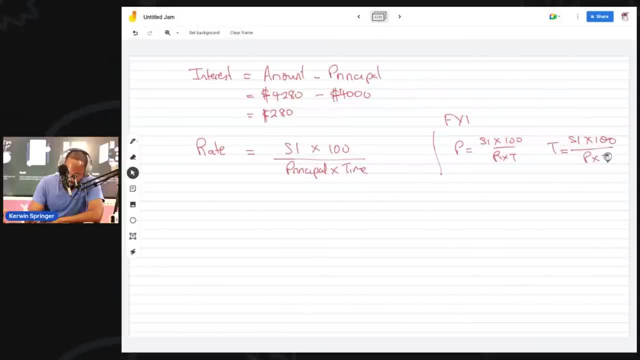 principle by time, by by rate, because time is already there, so we just need to substitute. the simple interest is um on the video and maybe you could take a screenshot and share it on your social media every day for the next two weeks. i want to try this lunch time between 12: 12: 30. we're going to come on. 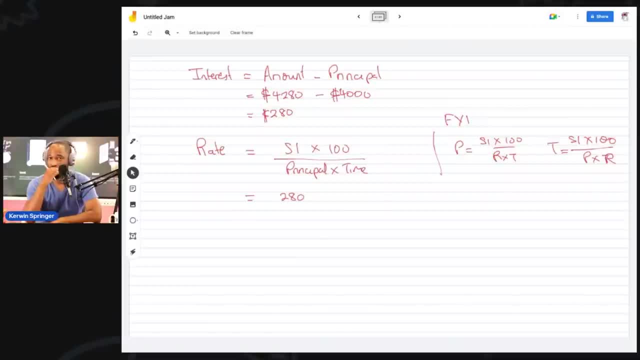 and we're going to do some studying right. so right now we just study in question one. the more you're going to study algebra, question twos. so if you're getting problems to study, come study with me, man, come study with me. multiply by 100 over the principal was 4 000. 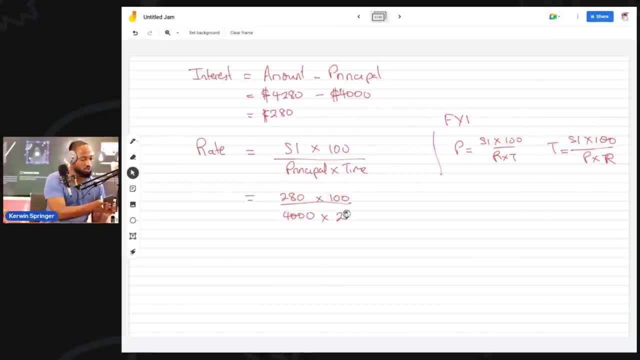 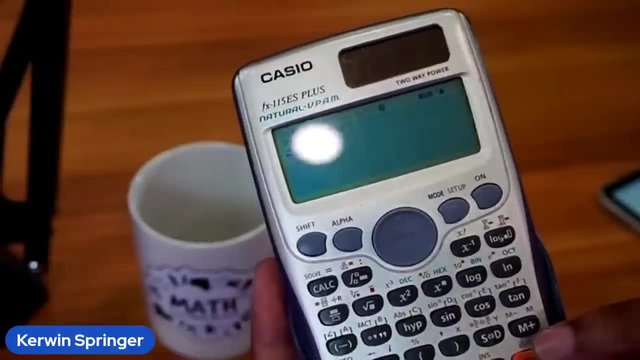 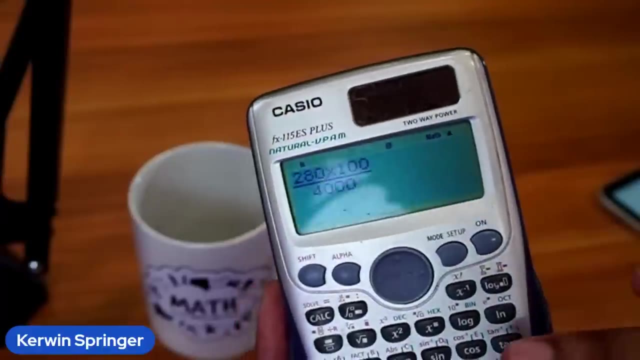 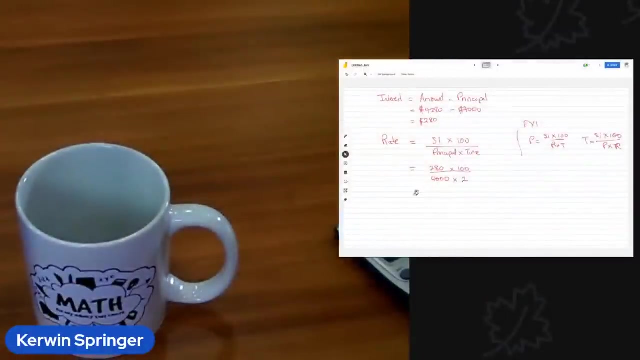 multiply by the time is two years. so let's, let's get the camera on the screen there. 280, i want to multiply by 100, and then i want to divide by 4, 000, and i'm multiplying this by two. oh two. seven over two is three point five percent. three point five percent. how many? 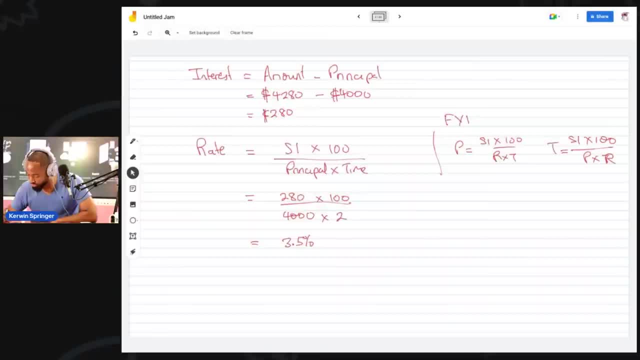 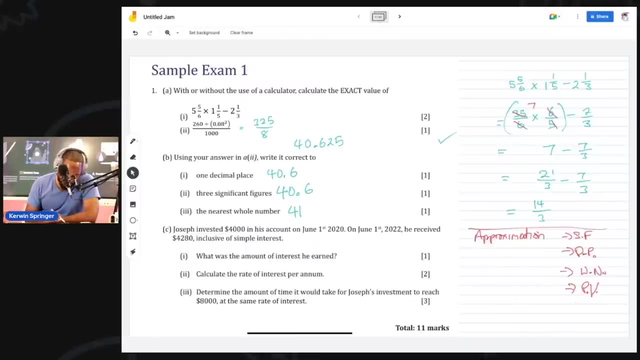 have you all got that? three point five percent, so last part of this question, and then we'll do another question and we'll see how much of this i can do before i realize i had to go and do some work. i have a stockpile out, so, um, what's the last one? determine the amount of time it will take for. 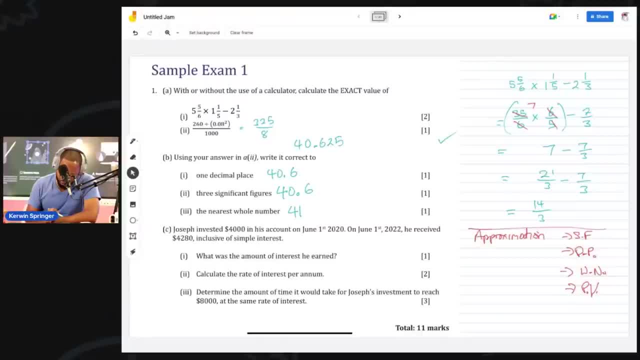 joseph investment to reach 8 000 at the- i thought i was the highlighters, i just scratch up my whole thing- at the same amount of time it would take for joseph investment to reach eight thousand. at the same interest. so, at the same interest, we want to determine the time, so we're just going to apply a. 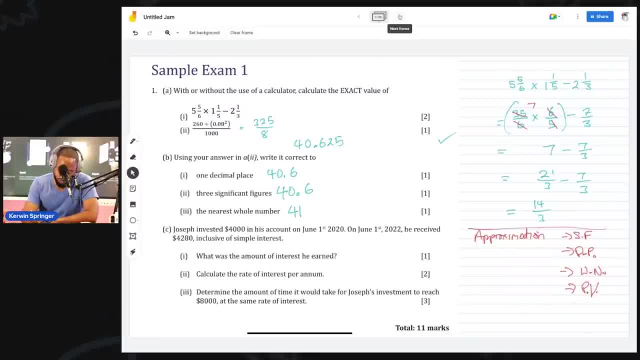 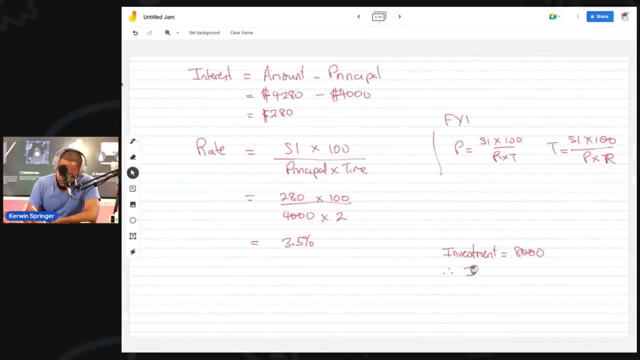 little time formula here, um knowing that if the investment reach four thousand, um eight thousand, the investment equal 8,000,. what's the interest Therefore? the interest is the amount, the investment. the amount 8,000 minus the 4,000 is 4,000.. So, with this new interest, the 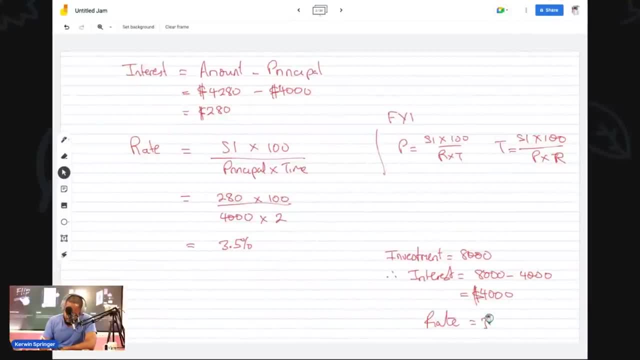 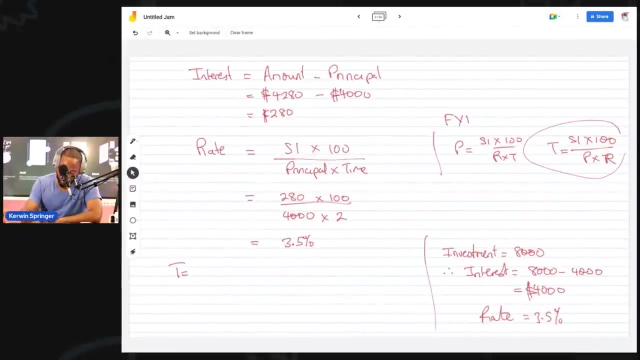 same rate. the same rate is 3.5%. We want to work out the time, So excuse me. So time is from this. simple interest times 100.. We're on page two right now. right Yeah, Simple interest times 100 over P by R. So the interest is not 280.. No, it's just 4,000.. That's a. 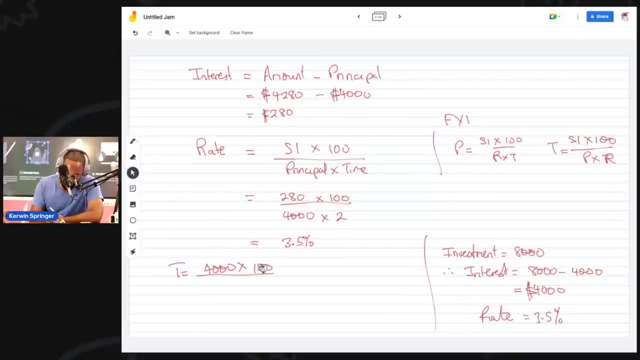 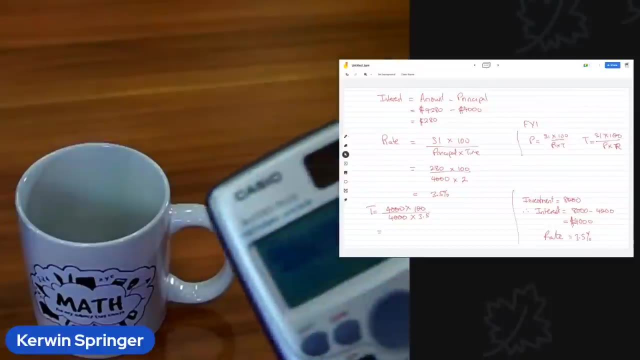 lot of time. this is going to take Times, 100, over 4,000 times rate 3.5.. And on our calculator put that. Put that in the calculator and tell me if you get 28.57.. If it's looking blurry, if. 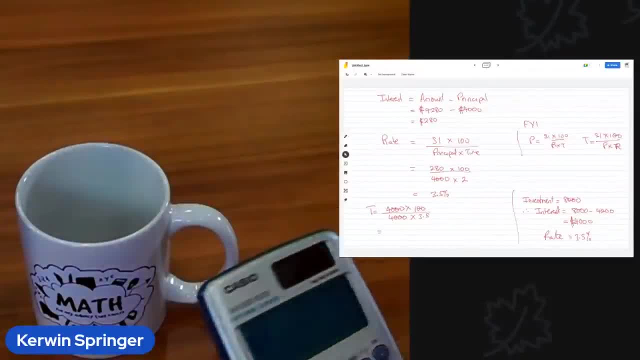 it's looking blurry. you need to raise the. So I'm seeing that 4,000 already. Cancel it 4,000 here. I'm seeing that 4,000, canceling at 4,000.. So it's really just 100 divided. 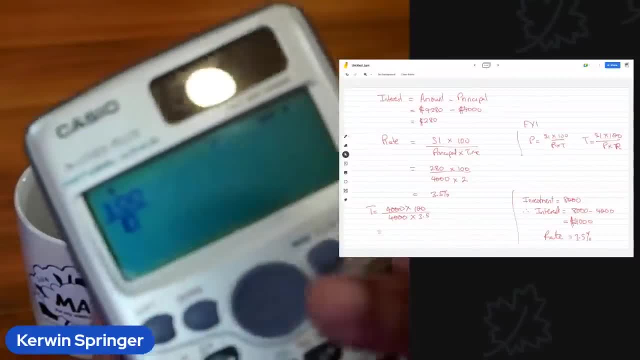 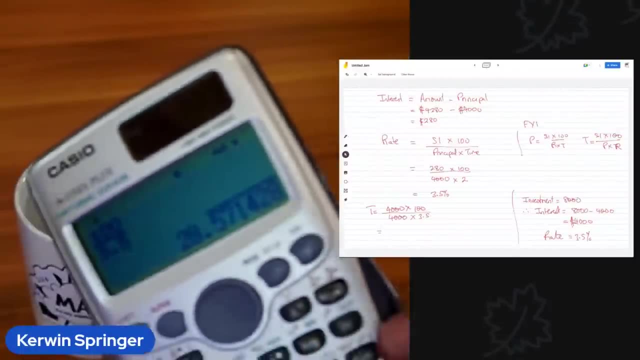 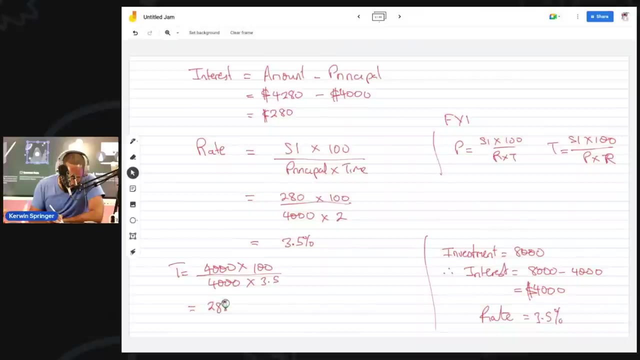 by 3.5.. 100 divided by 3.5 is 28.57.. 28.57, class. Are they getting that 28.57.. So we're getting that 28.57.. Now in the exam I can't say 28.57.. The interest is compounded. 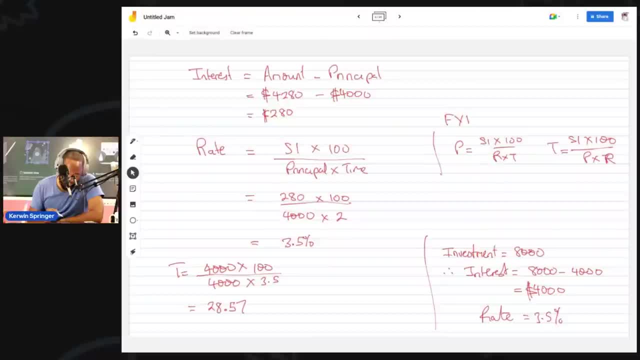 annually. You could see that here, Not compounded, added annually, because they actually give you some dates to work with as well. So only at the ending of the year it will cross. So at the 29th year we would. 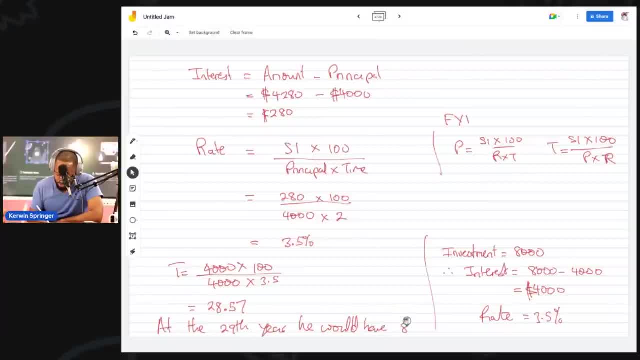 I have 8,000 plus in his investment. I ran out of space earlier in his investment. So most of the times with these simple interest questions, although you see a decimal- even if it was like 28.3, you're always wronged up. This is one of the cases in mathematics. 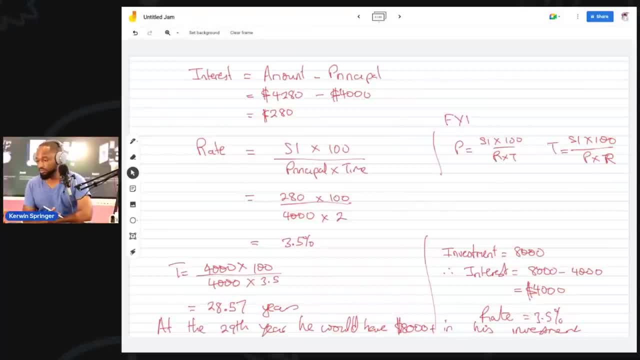 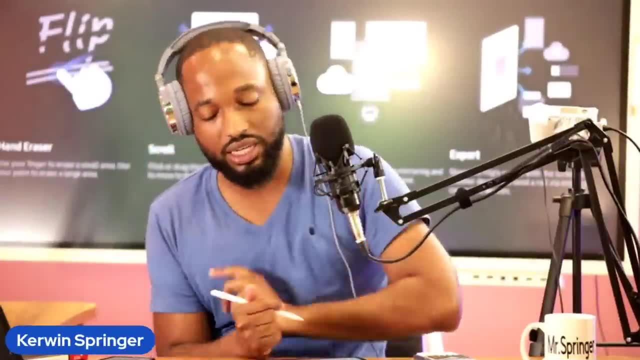 where you're always wronged up. So click these settings. Yes, Adriel B has it. Click these settings and choose 10.5.. Choose 10.5 and send that up. So let's do our next question one. I'll just give a little. 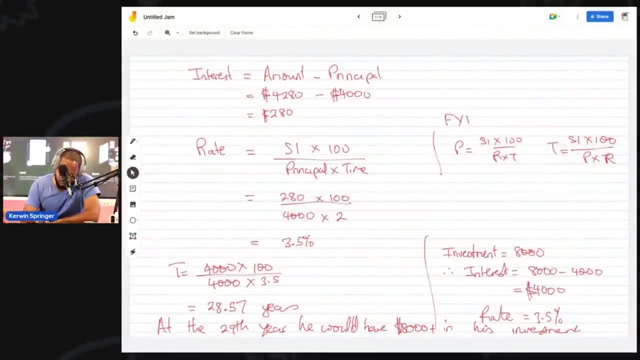 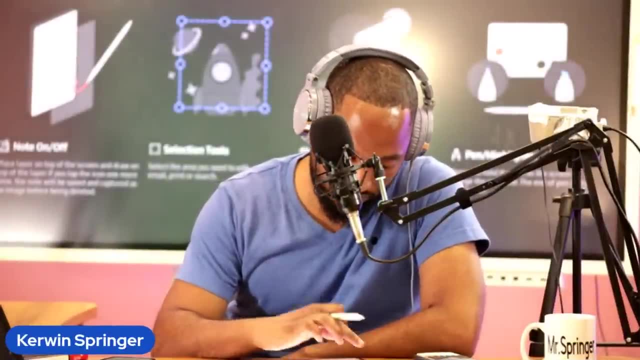 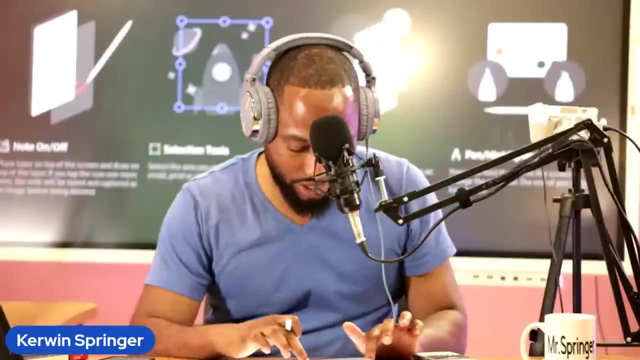 second, to bring up this question. one here, boy, Where did I put it? So these questions that I'm taking are from, And page three here trying to fight it up with this thing. here, boy, These questions that I'm taking are from this book. It's called The Question. 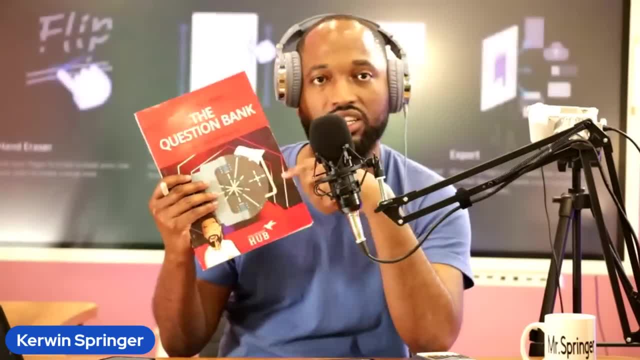 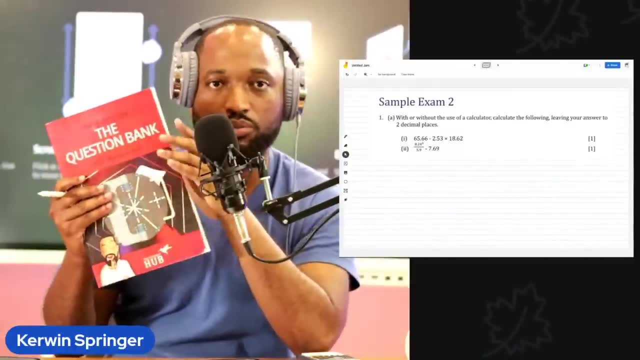 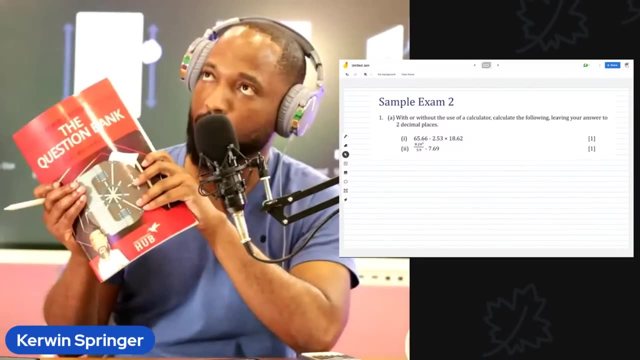 Bank And in this book I have all the usual multiple choice that CXC brings And I have five sample people based off of like the last set of exams. So it's like a prediction on what comes in the exam. So I'll try to update this book every year. My students, most of them, would 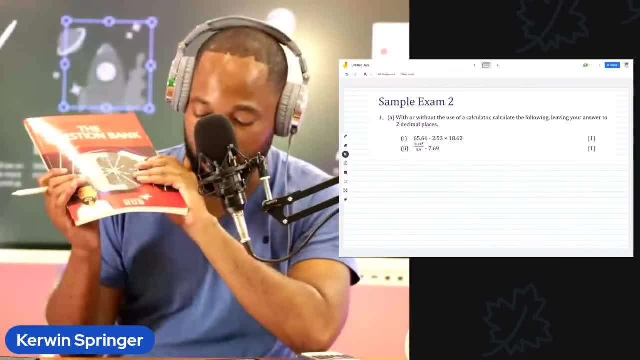 have gotten this book already, So it's an ideal preparation for the exams. The Question Bank: It's for CSEC mathematics And it's by written by yours truly, CXC. So it's a question bank: It's for CSEC mathematics And it's by written by yours truly, CXC. 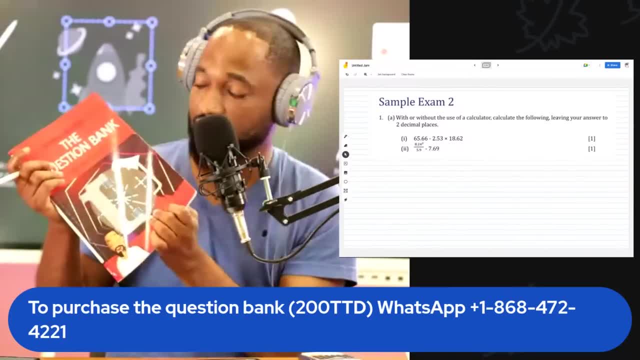 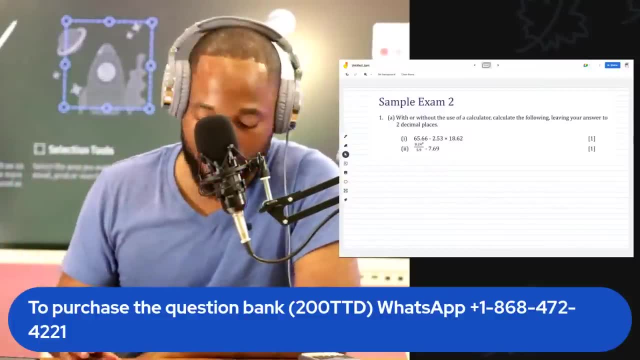 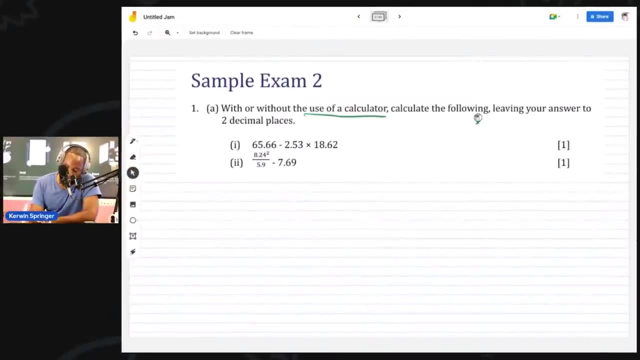 If you're interested in getting this book, it could be delivered to your Doie Phillipine insured And you'll just WhatsApp that number below there. So let's go. How do we do this question With or without the use of a calculator? Calculate the following. Leave your answer. to two decimal places. This is the key. That's the key. So the key here is that we're going to two decimal places, Just making sure my highlight is showing the Yeah boy Highlighter. All right, So that's it, guys. This was a very helpful question to answer And I hope. 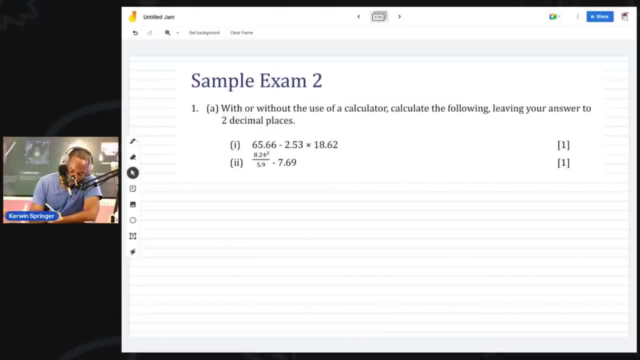 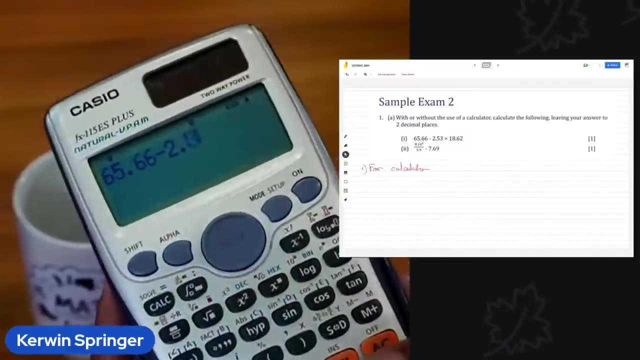 you have enjoyed it, Thank you. So put this in your calculator and see what you get. So from the calculator for part 1, real calculator use flying in here: 65.66 minus 2.53 multiplied by 18.62.. 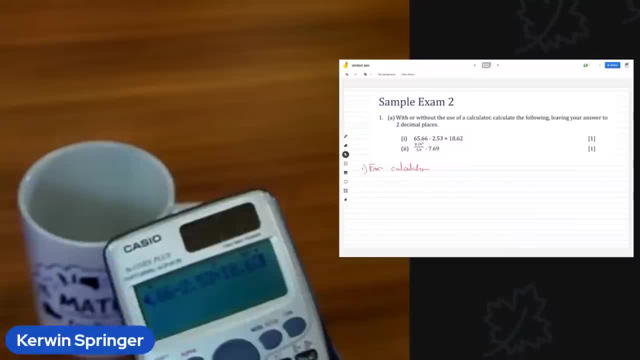 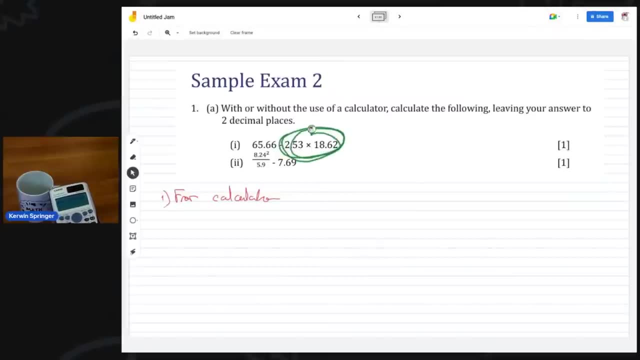 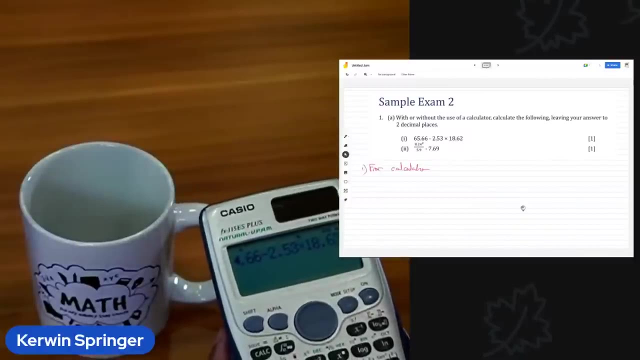 Now this calculator. this calculator knows back to the page. this calculator knows to do the multiplication first, So it operates it by mass in mind, But you could literally type it in, just so, and, as I said, the calculator knows. So if you're feeling a little jumpy about that, you may have to use brackets right, Especially those with not this calculator. 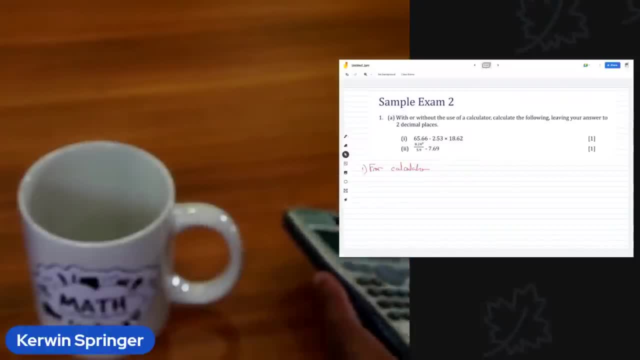 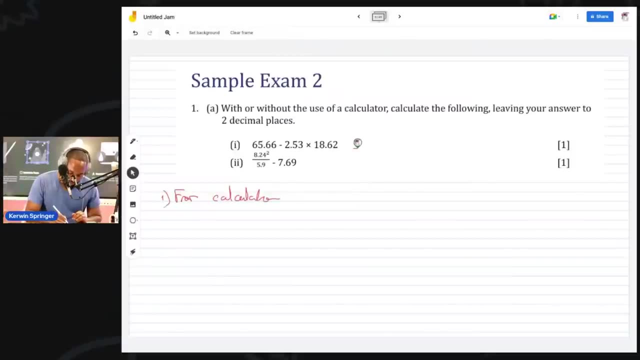 And 18.55 is the answer. Is that the answer? we are getting 18.554?. How many of you all got that? From the calculator I'm seeing 18.5514.. So, to two decimal places, it's 18.552, two decimal places, And the reason being the two decimal places not greater than five. So I don't need to give this a booster, I don't need to give that one a booster. So let's get the other one one time and collect remarks and go. 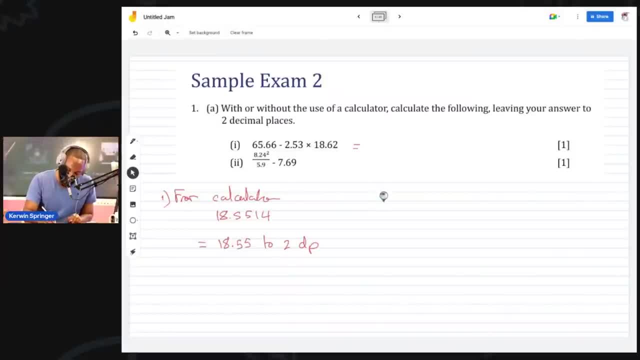 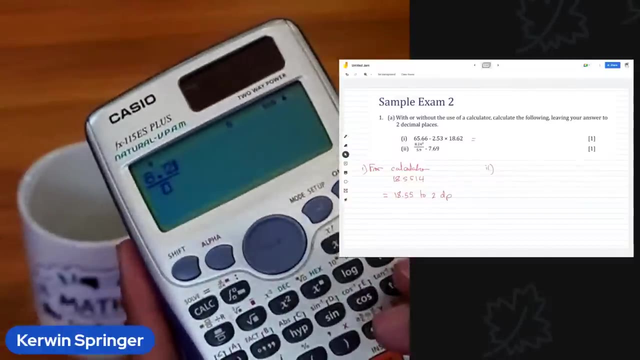 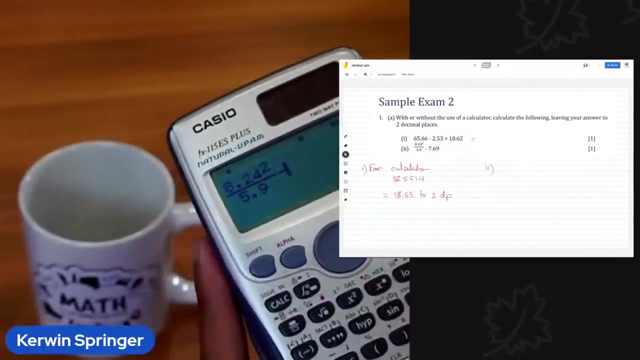 So easy questions we're starting off with here Next, And I'll see you next week, Tomorrow, please go, I'll be doing algebra. Tune in for that. Tune in for that. It's a very important session. Let me jump back in the calculator Calculator: 8.24 squared over 5.9 minus minus 7.69.. And we get one long number. 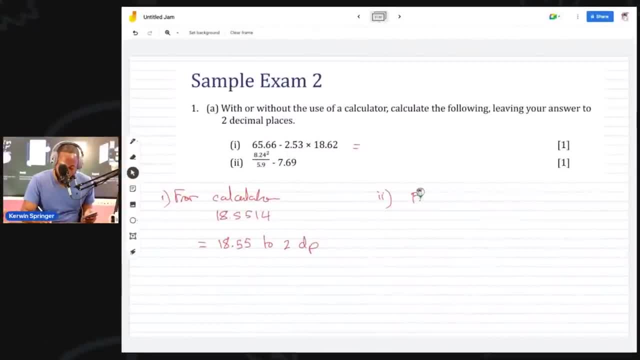 So from the calculator I got 3.818067797.. One step back now, But two decimal places it's 3.81.. Hey, no, it's actually 3.82.. Now why is it 3.82? Easy thing. 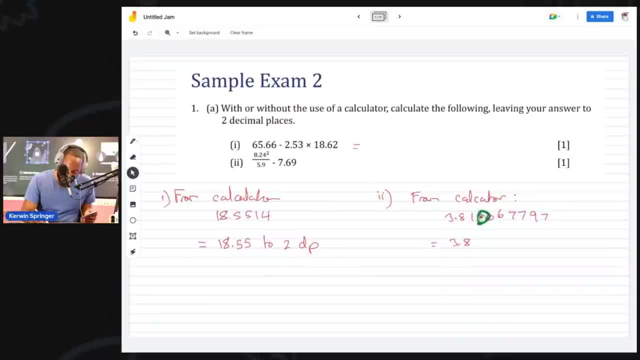 That number. that number is greater than five, So you have to come here now and get that one a boost. The car boost is different: Two decimal places. So easy stuff, Easy stuff. Let's go on to the next part of this question, which would most likely be consumer arithmetic. 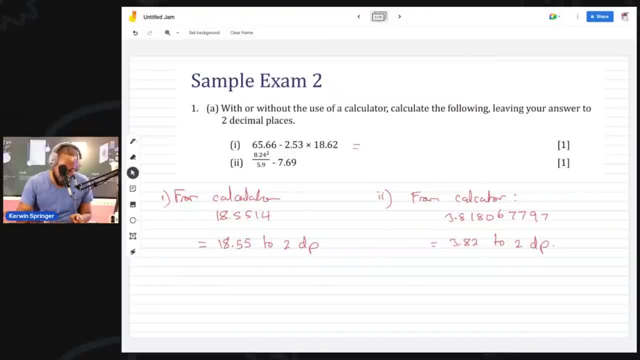 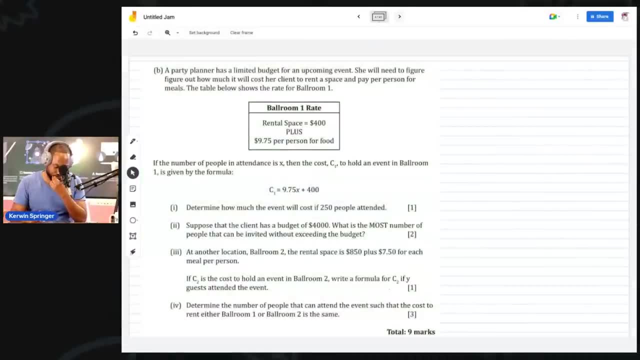 That's a big consumer arithmetic question. Let me know if that's too small. I'm on page four here. Let me know if this is good enough for you. So and this question I'm seeing. I'm seeing something about a rental, something about food and then an equation. 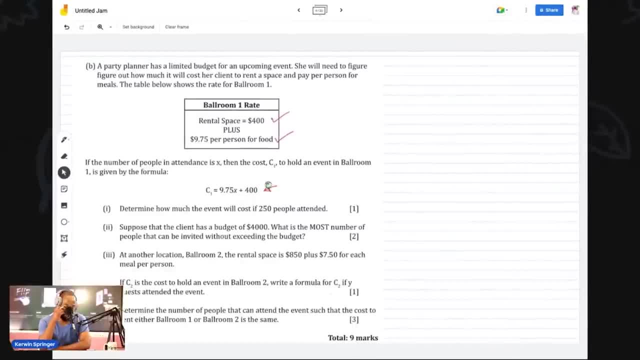 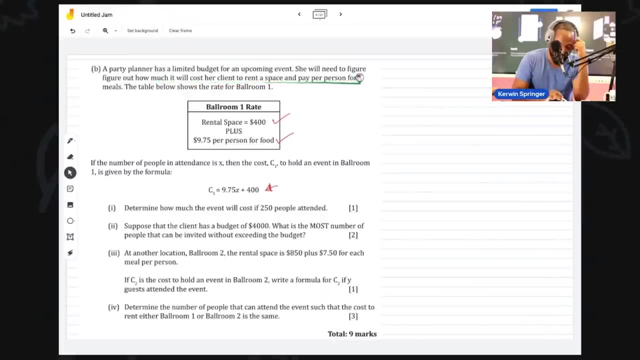 So they have been doing this weird thing recently by CXED, including algebra in the first question, the consumer arithmetic question. So let's read the question. We have a party planner limited budget. You will need to figure out how much it will cost a client to rent a space and pay per person for meals. 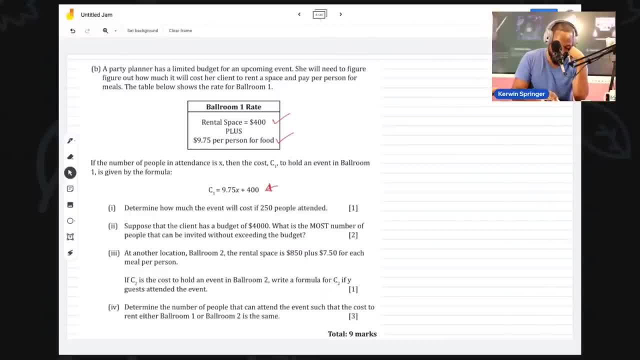 The table below shows the rate for ballroom Ballroom one, Or bring in a ballroom two later on, any question. So you have to pay the rental space and then $9.75 per person for food. So it's really the rate, the standard fee, the fixed cost, the constant plus X is the number of people by the cost of one person for food. 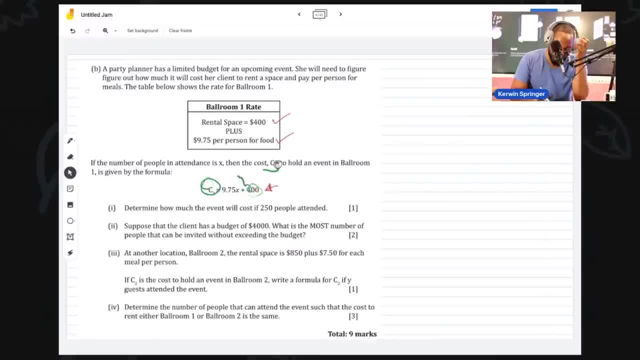 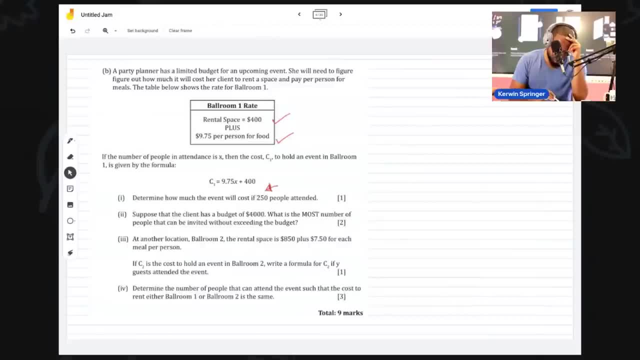 Why is it in the chat if you don't understand what's happening? That's the cost to hold it in ballroom one, Beautiful, Beautiful. So suppose the client has a budget of $4,000.. What is the most number of people that can be invited? 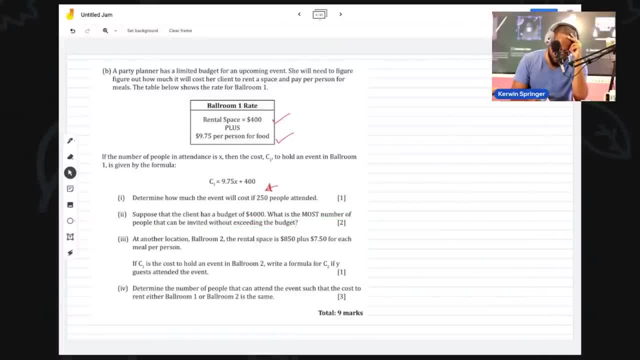 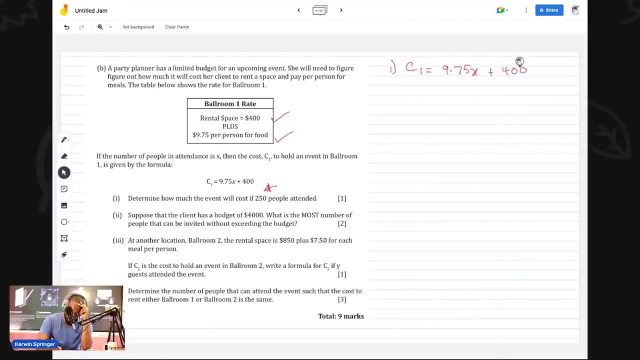 Number one determine how much the event will cost if 250 people are invited attended. So C1, for part one, C1 is equal to 9.75X plus 400.. So if X is equal to 250 persons, 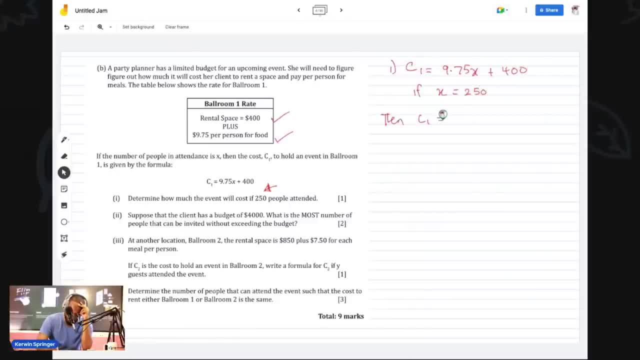 then C1 would have to be 9.75 by 259.. I can't be calling me now. I'll have to take this call. Leave my wife, Thank you. Yeah, earlier that was CXE, and CXE calls to say good job. 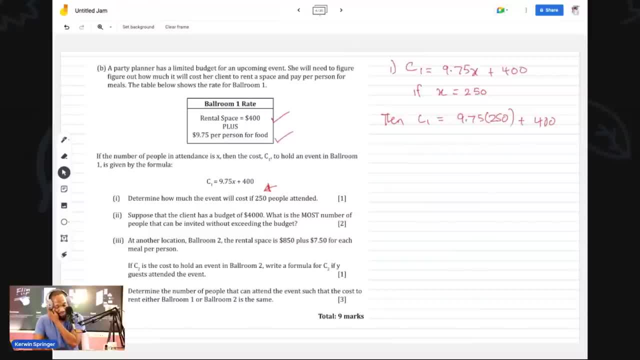 It was, it wasn't, and see it, And CXE would never call me and say: good job, All right, so 9.75X by 250.. CXE would never call. call me 9.75X by 250.. 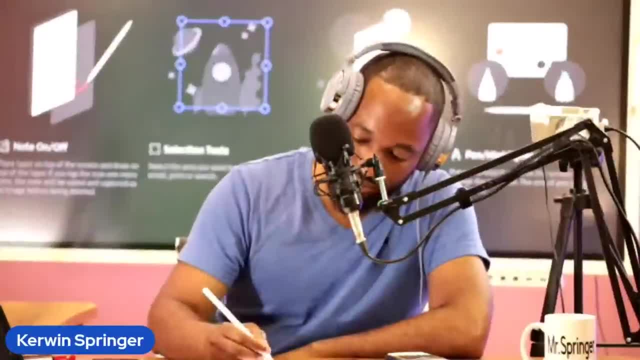 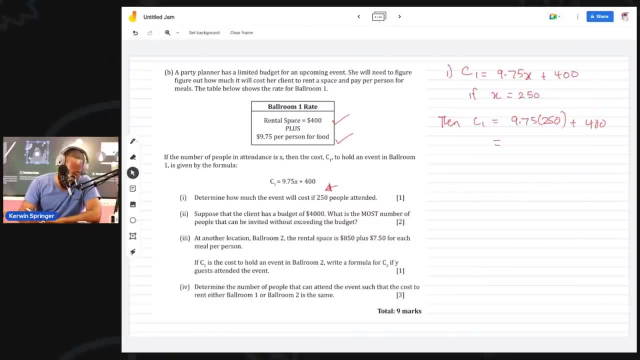 CXE 9.75X by 250. CXE calls these heaters plus 400. what do y'all get for this? 2937.50. isaiah. isaiah is sure about that way. i, like anybody else here, different answer. i get two, eight, three, seven point five zero. 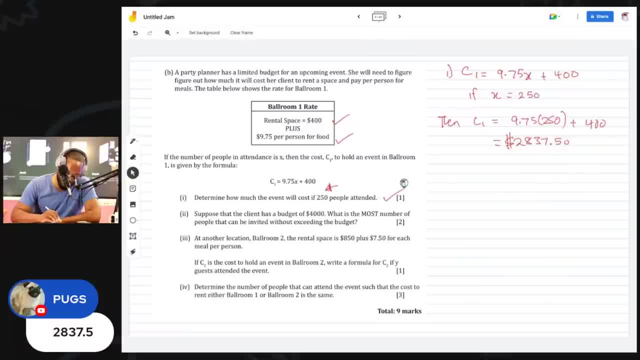 so check it over. um, so that was one mark, and suppose the client has a budget of four thousand, what's the most number? so, uh, for part two, it's setting up like an inequality, but you could work it out even if you didn't know to set it up like an inequality. what you're trying to see is that. 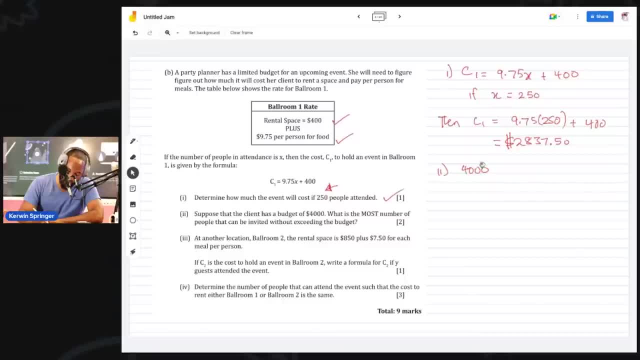 four thousand. um, whatever we have here must be less than or equal to four thousand. so nine point seven five x plus four hundred must be less than or equal to four thousand. so if i bring across the four hundred on the left hand side of the equation, or the inequality um, i would have nine point seven five x here just remaining by itself. 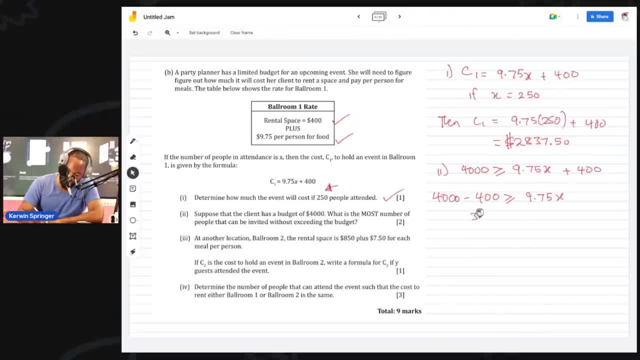 and four thousand minus four hundred is to the six hundred and that's nine point seven five x. so i really just need to divide to the six hundred by nev, by nine, by nine point seven, five, right to kind of zero in on that x value. and if i do that, how much am i getting? i'm going three, six. 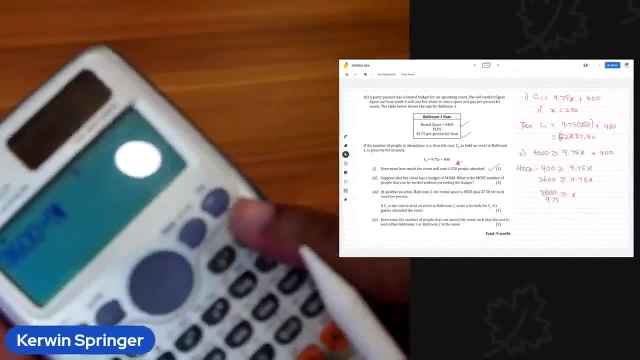 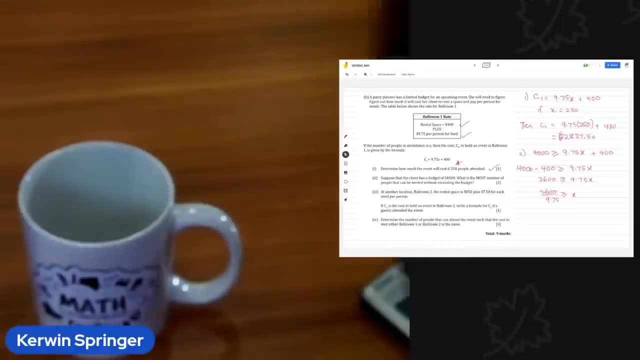 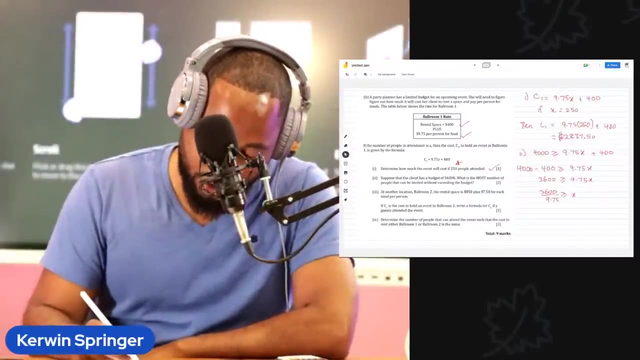 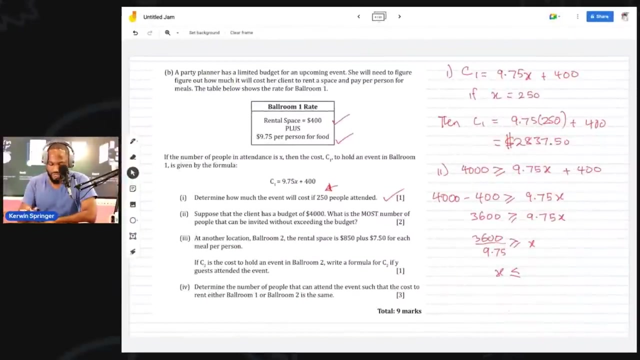 zero zero divided by by nine point seven: five equal to four. eight zero zero over thirteen. so i'm getting um. now i'm gonna do a kind of switch around here, but if i swap left hand and right hand side, i need to excuse me. i need to flip the inequality sign right. so this is three, six nine point two. 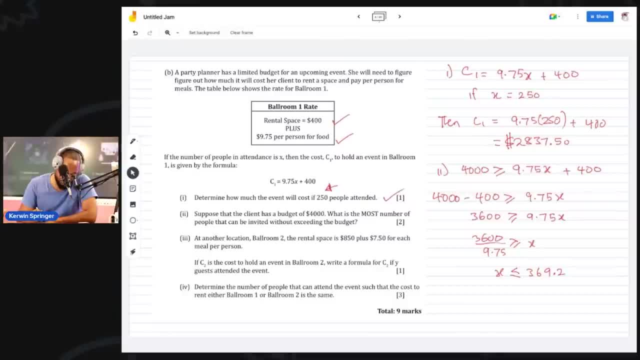 so because we notice the most number of people that can be in invited, because we can't have, we can't have half a point two of a person, we need to say: well, x could only be 369, so how many of you all get 269, therefore the least number. 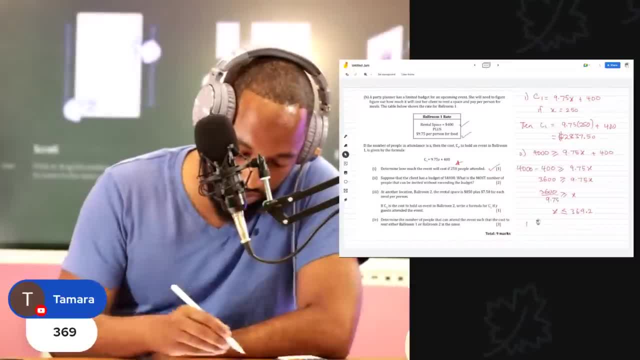 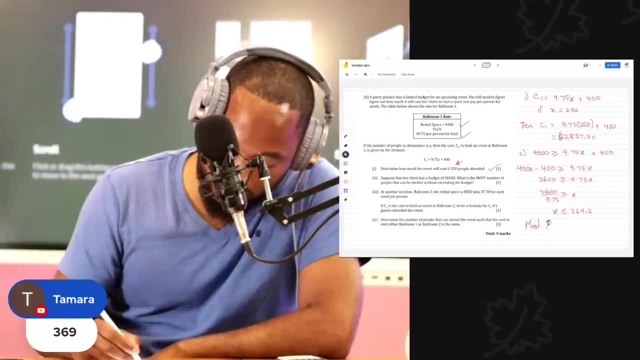 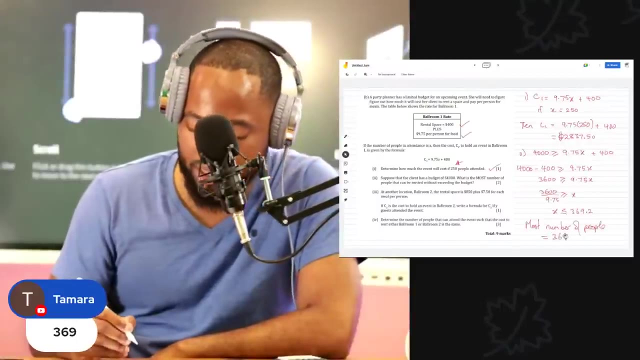 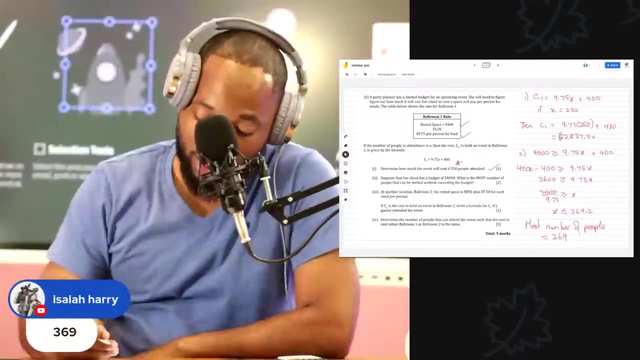 or the most number, sorry, most, what's the most number of people has to be equal to 369. if i go over, it will go over 4 000.. if i go, 370 though. so this is one thing. okay, january, you always need to round down. even if this was 369.999, i still need to say 369. i can't. 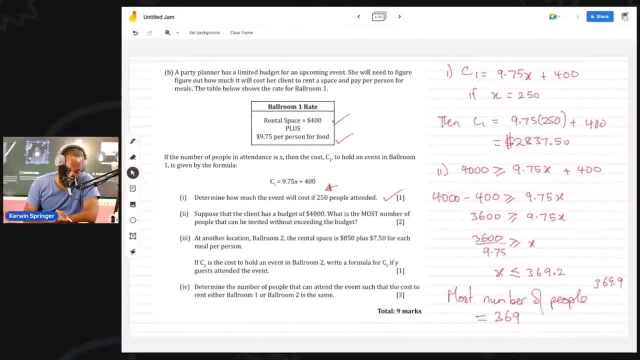 say three hundred and six, three hundred and seventy, because i i would go over the four thousand. so make sure you understand that for this i really want to make sure you understand that there's another part of this that needs to be done. let me see if i can get on page five. 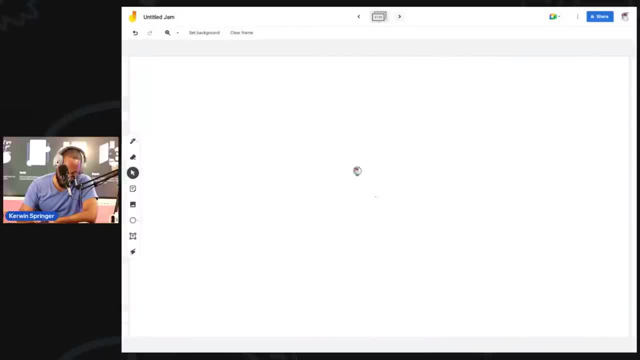 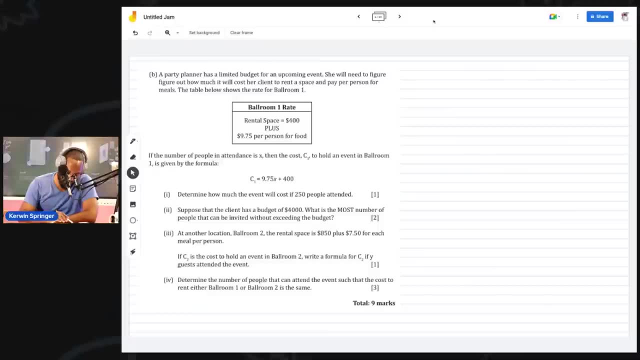 and set the background for page five. so on, magic five now. all, right now, finish this, finish this. we just need to collect with four more marks and go. only want to do one more question, one after this, one more, two more, three more. how much more come any more question? 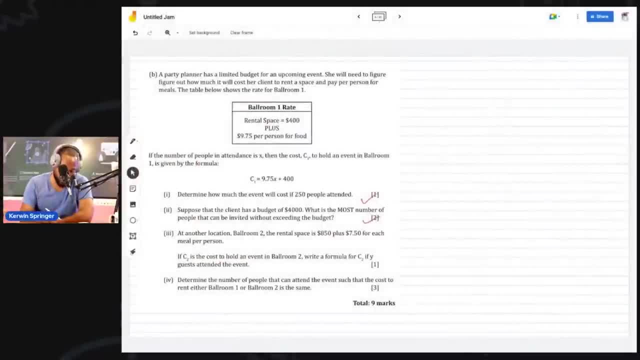 once y'all feel we could do at another location. volume two: your rental space is 850 plus 7.5 for each. write the formula. so the formula will be: c2 is equal, just like this formula, and instead of x we use in y and the fixed fee. how much is the fixed fee? 850, also enough, and it's instead of: 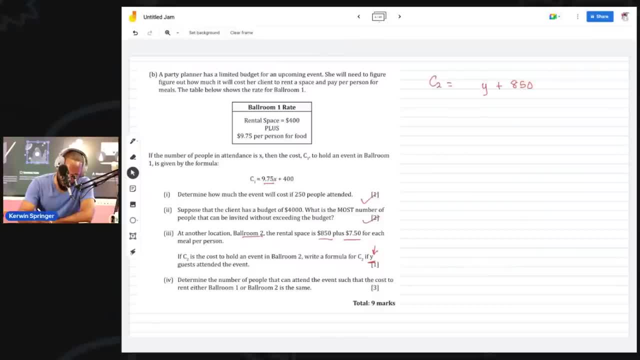 instead of it being 9.75 for business, 7.50, so 7.50. how many of y'all got that nice, nice, nice. two to three more. two to three more, okay. so we did the formula. you see, many number of people that can attend the event, such that the cost to 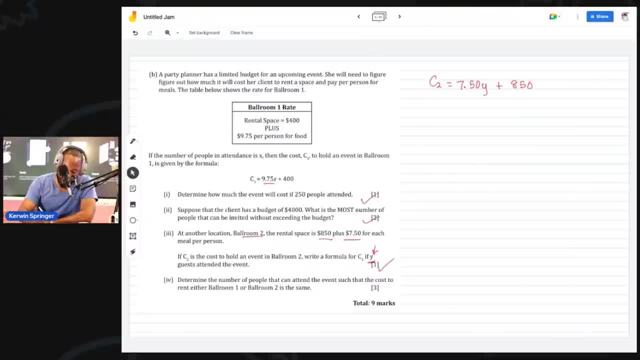 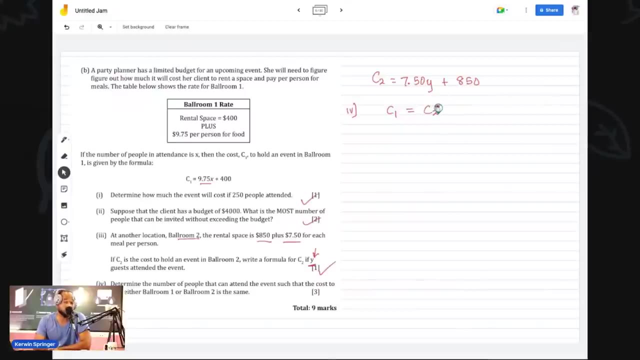 rent. either volume one or volume two is the same, so we want c1 to be equal to c2, for y'all understand. that's what they're asking for. part four: that's a straight up algebra move. i was predicting that that would have happened. i was feeling it in my heart and soul. when you do enough of these, 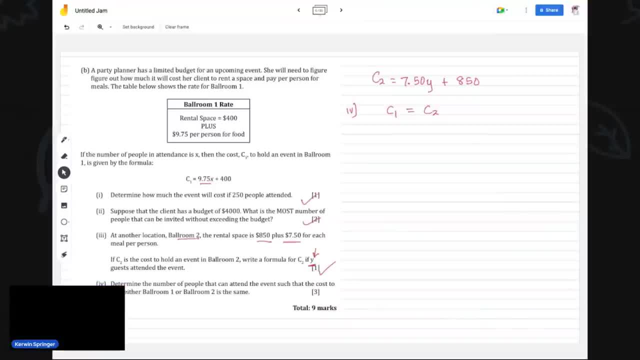 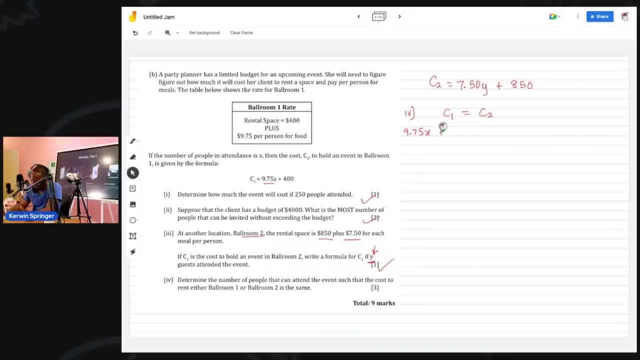 questions. there's no way they're coming from one time. so you want c1 to be equal to c2, but c1 is 9.75 x plus 400, is equal to c2, which is 7.50 y plus 850. but in this situation we want. we want c1. 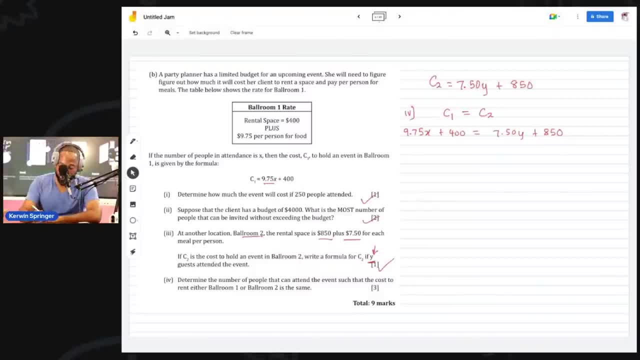 to be equal to c2, so therefore the number of people will be be the same. so in this case x is really equal to y. so i can rewrite this equation and i'm going to do the same thing as 9.75 x, and then plus 400 equals 7.50, but instead of putting y i could just put x again. 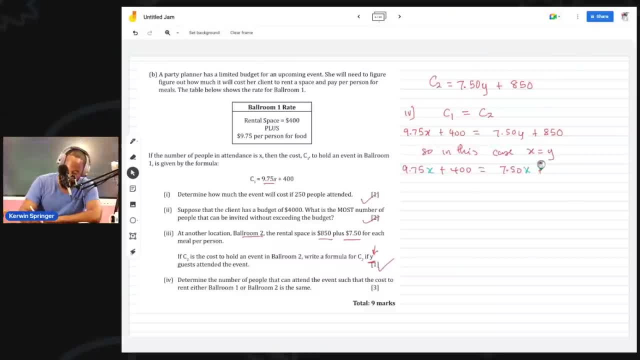 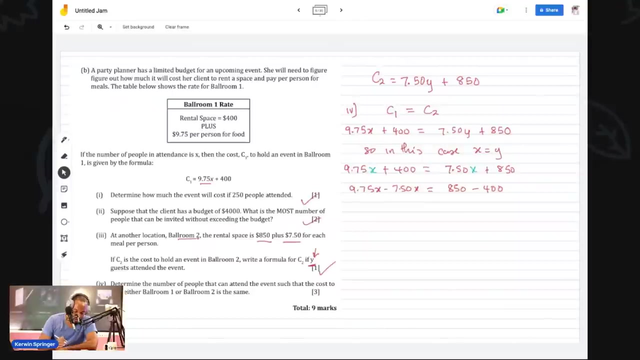 plus 850, and now it's just to do some little swappy swaps and see what going on there, right? so if i switch around everything you should understand, i'll have 850 minus 400 and then i'll have 9.75 x minus 7.50 x. so 9.75 minus 7.5 should give me 2.25 x, and 850 minus 400 should give me 450. 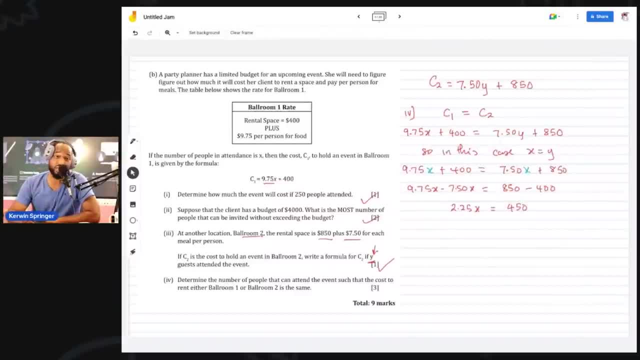 you going good so far. why isn't the chat if you're following everything in this life? and then, finally, x should be equal to 450. hopefully, get a whole number over 2.25 and it's exactly how much you'll get: 200, 200 persons. 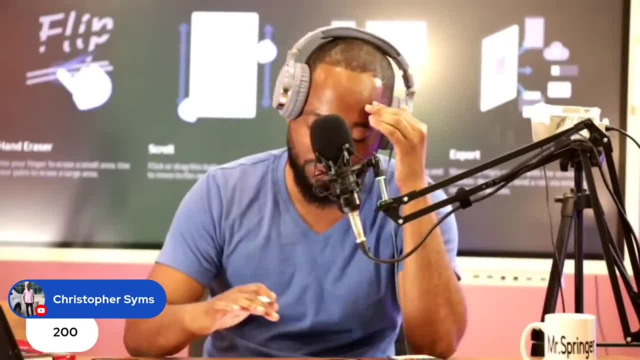 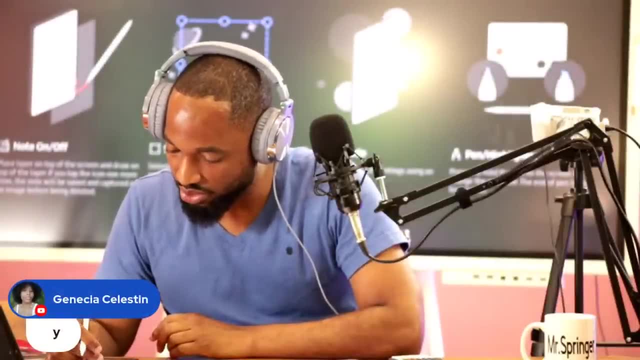 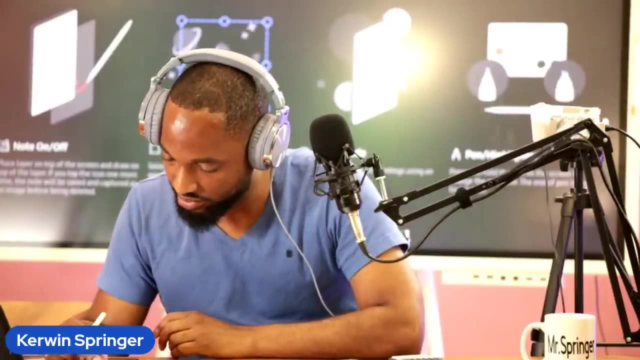 and we finish this question. so you all say two, three more. let's see if i can squeeze in one more. just give me a couple seconds to grab this, people. how the revision going. how the revision going. if your revision was a, was a movie, what would be the movie title of your revision? 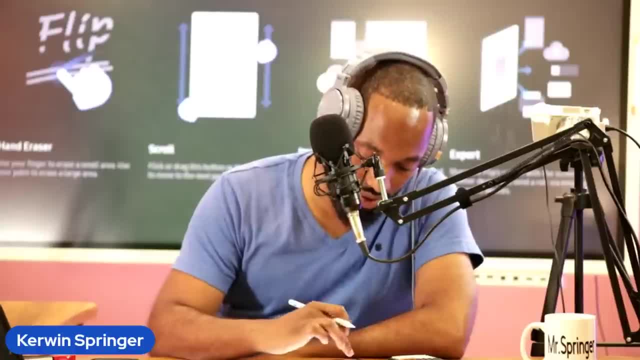 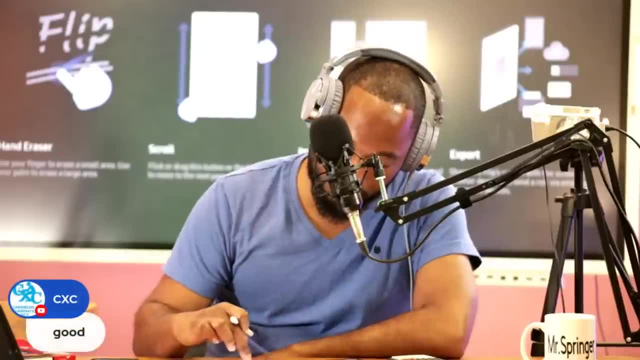 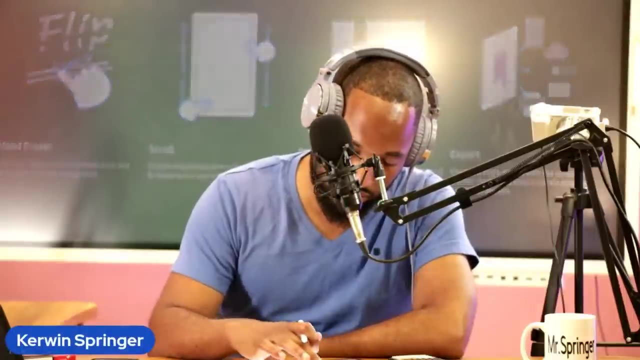 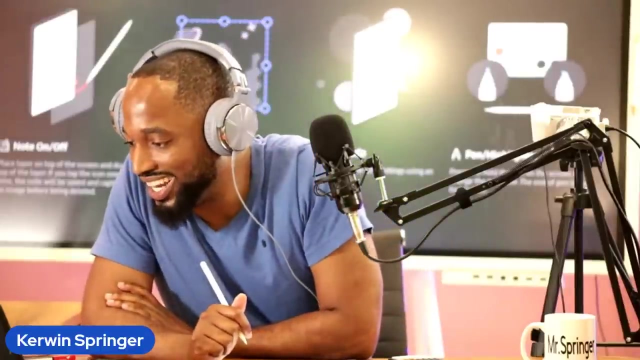 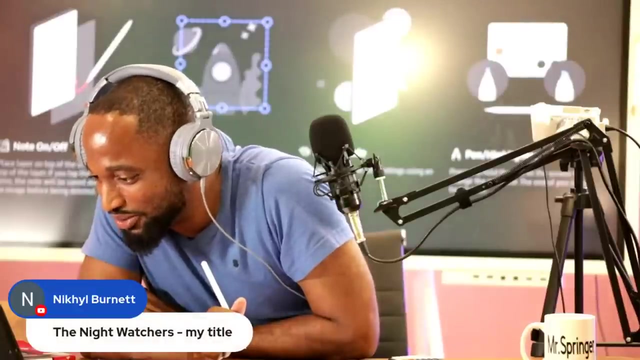 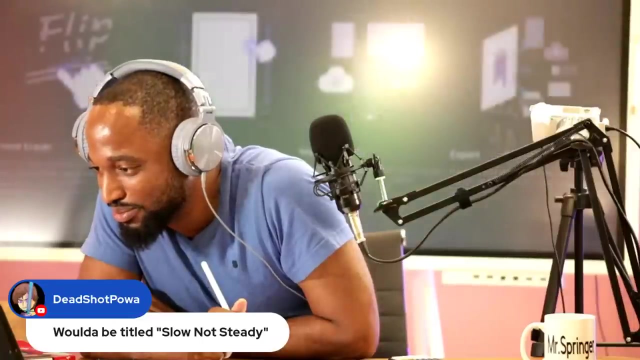 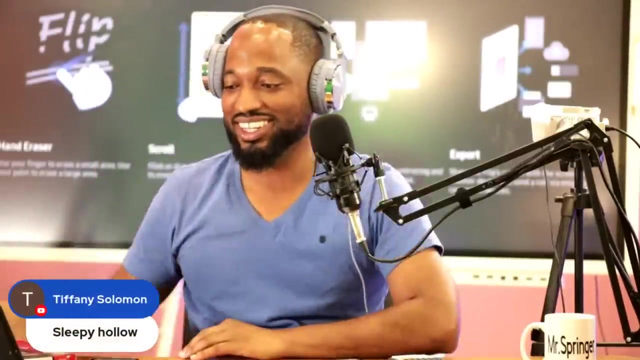 what would be the movie title of your revision. so on slide six here, let's see if we can get a background. nice six, the night watchers. titanic zootopia will be titan, slow and steady. titanic scream black race. it is mission impossible. sleepy hollow. get smart, get smart and pass trying. 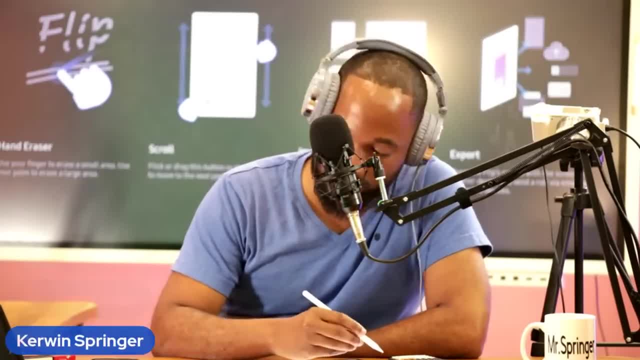 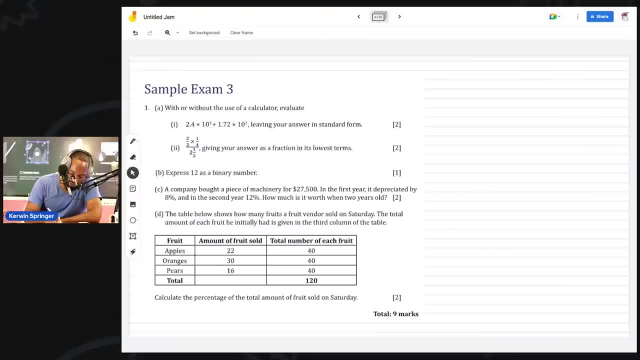 are they very creative, boy? all right, so with oh, we told you we have our next question here. we thought, without the use of calculator, evaluate this time. i like how we have differences, we have standard form and giving your answers a fraction into lowest term. and then, oh, we have a nice beautiful question here on binary numbers. 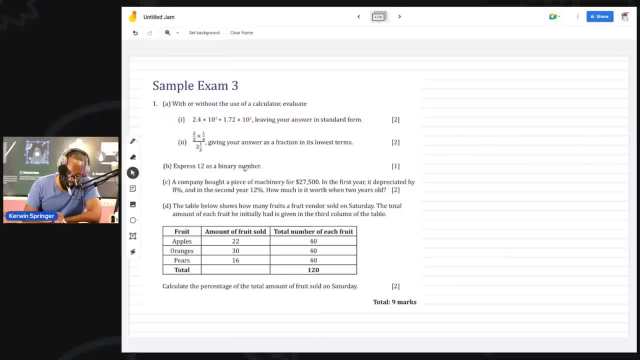 looking forward to doing that. we have a question here on depreciation, popular topic. and then what's this? we have a kind of um invoice question here, one of the invoice questions, and percentage: only two marks, two, two one. so this question is nine marks when you look in the exam. don't tell me my battery dead. 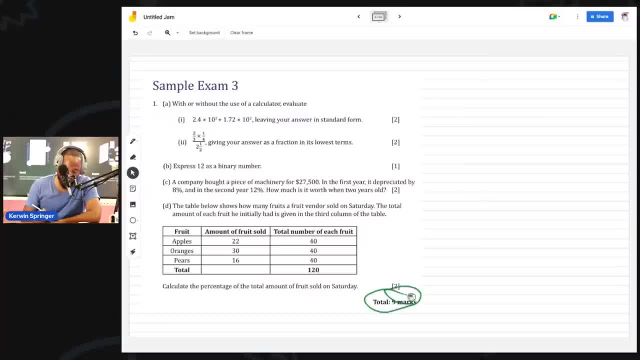 day when we look in the exam, you're gonna see nine marks for this question. so let me go, because if my battery dead party done, i might have the right with my finger. so 2.4 multiply by 10 to the power of three plus 9.4. 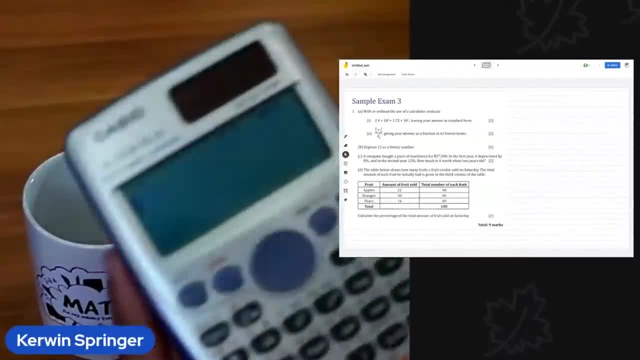 9.4, 9.4, 9.4, 9.4, 9.4, 9.4, 9.2, 9.3, 9.3, 9.3, 9.4, 9.4, 2.4. 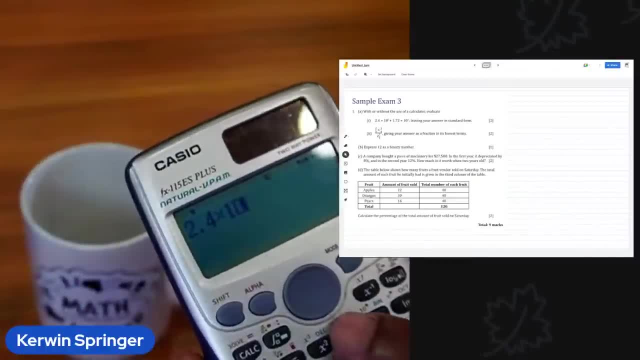 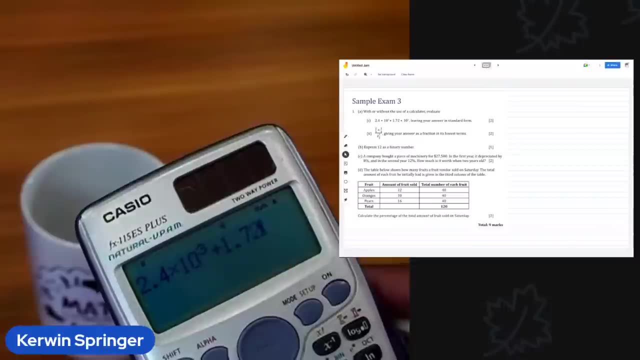 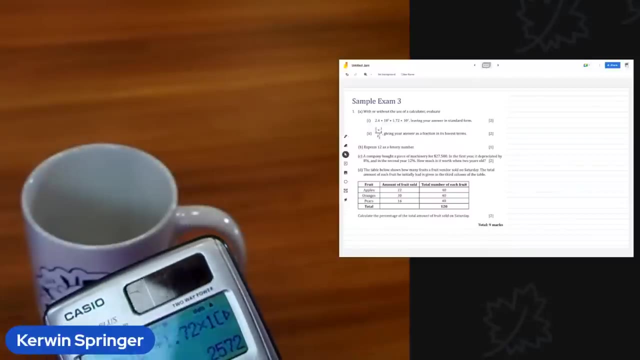 multiply by 10 to the power of 3. i'm gonna literally write it out. there's a way you can do standard formal. i'm gonna write it out: plus 1.72 by 10 to 10 squared. it's only calculated. my calculator is saying that the from from the calculator i am getting. 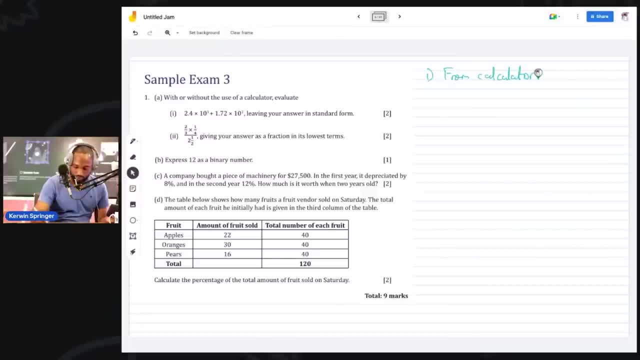 9.4, 9.4, 9.3, 9.4, 9.4, 9.2, 9.4, 10.4, two five, seven, two. but the answer must be in standard form. you all know how to take a number. 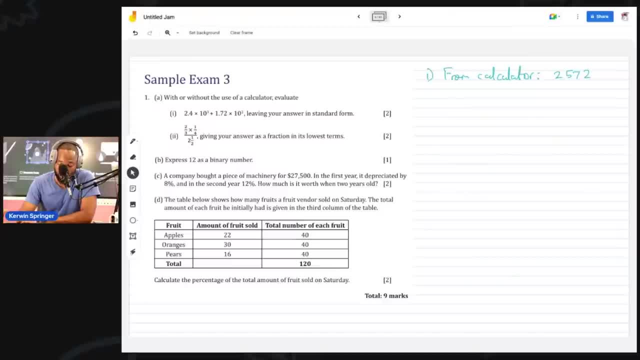 and change it into standard form. you all know how to do that. so you watch where the decimal place is. you move it just before the first non-zero number, which is two reading from here. it's two, so the decimal point must come right there and you record how many times you move it and since you're moving. 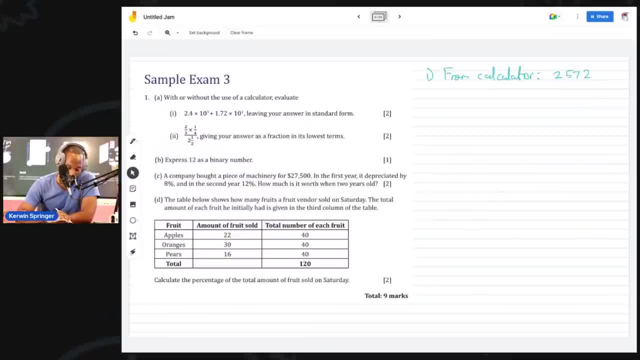 it to the left. it means the number is bigger than 10, right? so you're going to have a positive 2.572 multiply by 10. you're going to have a positive index here. three, you move it three times. why is it in the chat? if you understand that 2.572 multiply by 10 to the power of three? 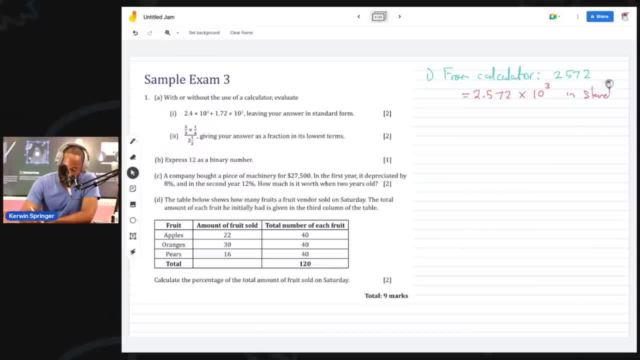 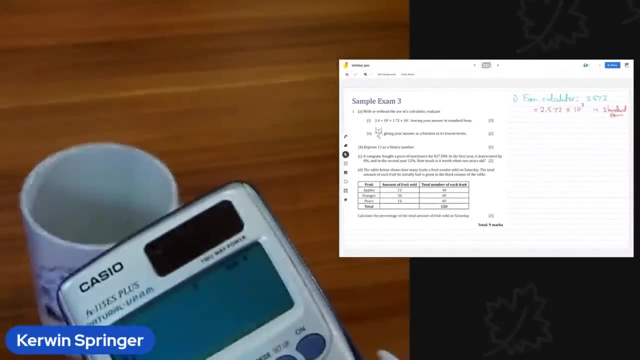 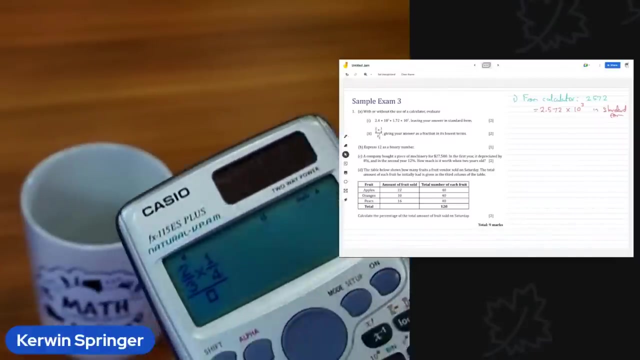 and that's in standard form. and now we need to give this as a fraction in its lowest terms. by the way, an improper fraction is still a fraction, so let's just type this up: one time: two-thirds multiply by a quarter. there we go. oh no, i didn't divide by anything, syntax error. so you see, i didn't press on, so 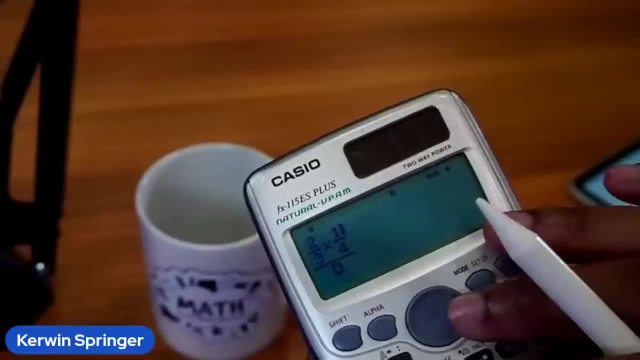 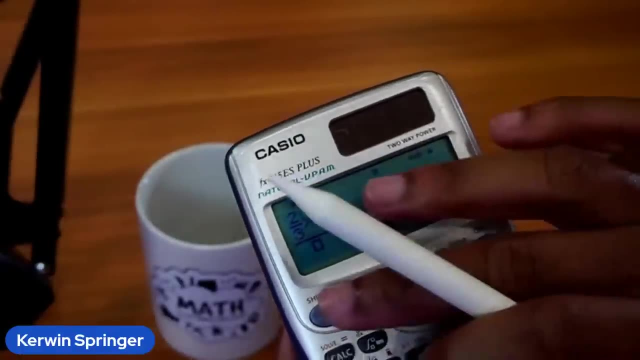 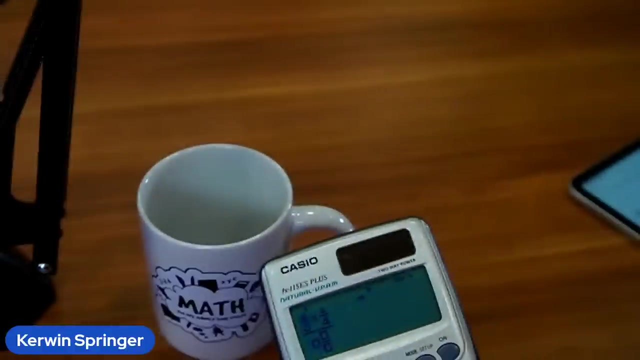 i can just go back and edit my stuff. divided by what? by two and two and a half. so there's actually. there's actually. if i press shift and then i press the fractions, i can get my mixed number. that's the only way to do a mixed number fraction. you can't manually put a number and then put a fraction, like wireless. 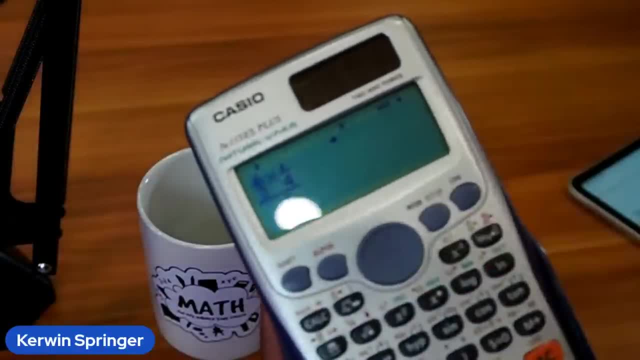 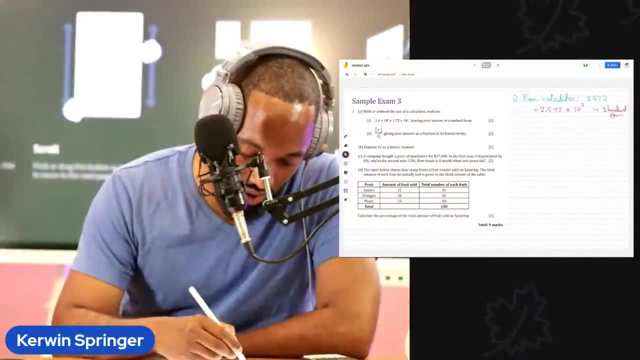 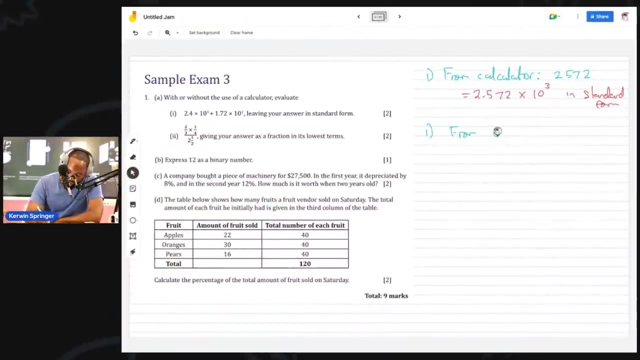 so two and a half bang 1, 15th. so from the calculator it's just straight up. got that now. obviously i would advise for this question to come back and show the full working, but for now Now I already showed you how to do the weekend and these kind of things, but now I will just. it was two-thirds multiplied by a quarter over two and a half. 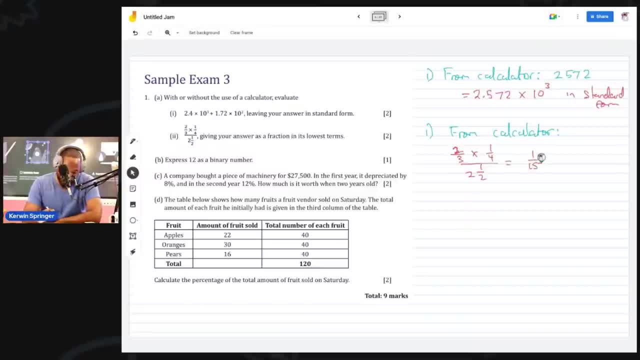 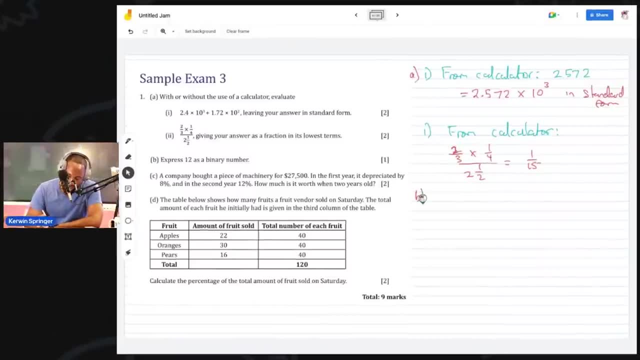 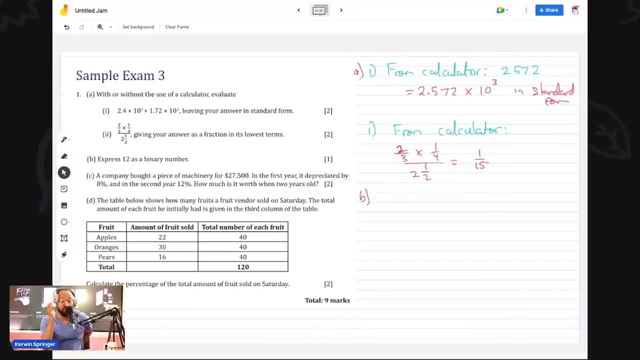 I will just put the answer straight up: one-fifteenth, So express 12 as a binary number. that's part B: express 12 as a binary number. So how do we take a number that is in denary format, decimal format, base 10, and change it into a number that's in binary format? 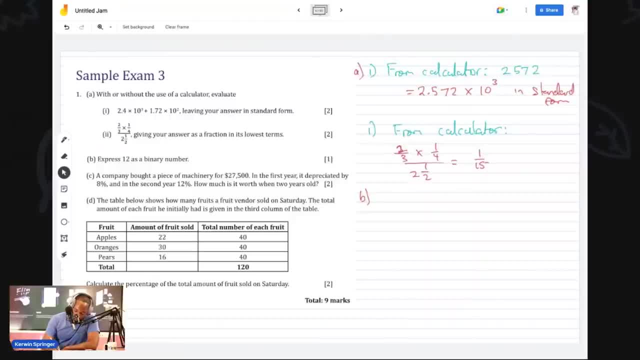 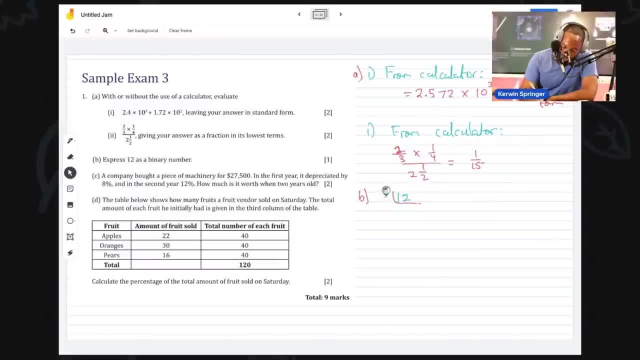 You all remember how to do this. You remember how to do this class, So you put the 12 here and you start to do a kind of breakdown thing here. But since you want to go into binary, you do two, Two into 12, six and you record the remainder every time. 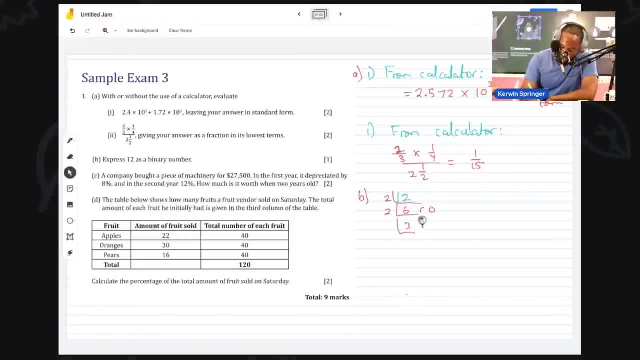 And then two into six, three- No remainder again. And then two into three. one, One is the remainder, My finger touching the screen and making these little dots down on the paper here, And then two could go into one. zero times remainder one. 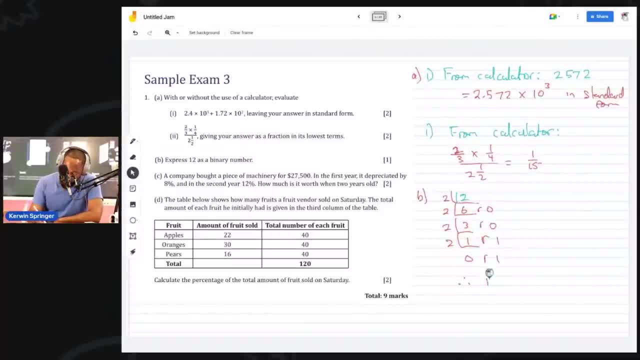 So the answer is therefore 12 base 10 is equal to- and you read it going up- is 1, 1, 0, 0 base 2.. As simple as that, And if you don't know how to do it, you don't get a one mark. 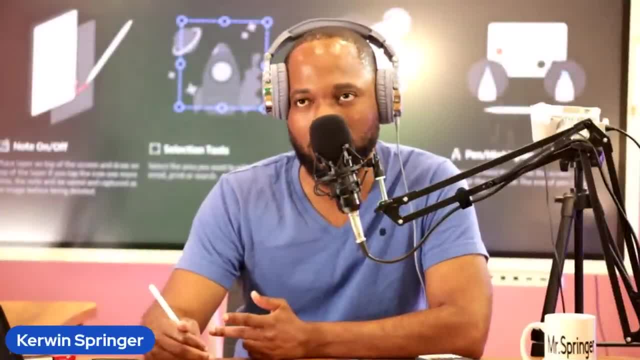 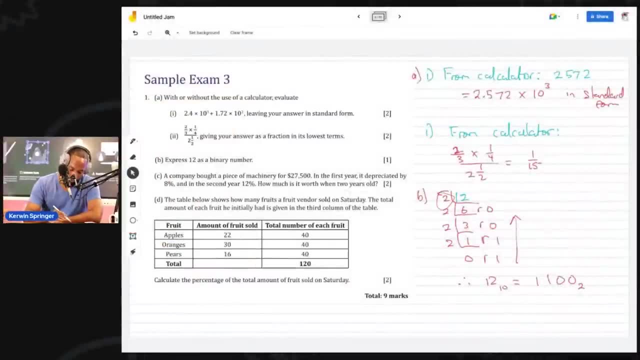 They ask this Maybe twice. They ask like seven And then they ask six. It is possible that they could ask a different base. You would just change your number here, right? Okay, Let's go forward. So where are we at? 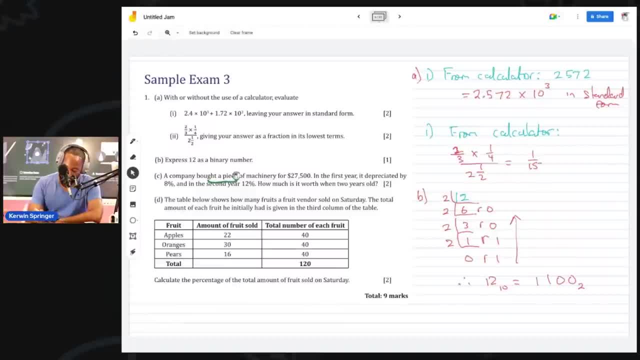 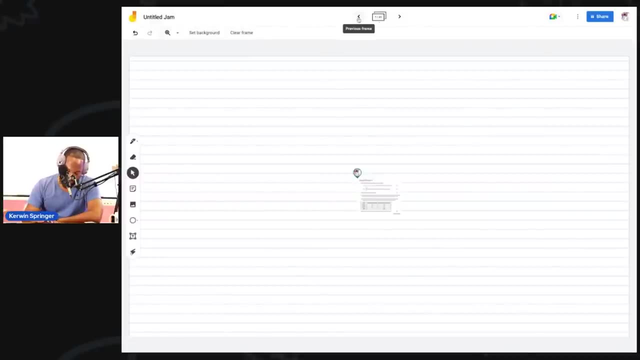 Four more marks to collect. A company bought a piece of machinery for this amount. Let's see. Let me go into the next slide and see if I can just post that part alone so I can get some more space. Where is this? There we go. 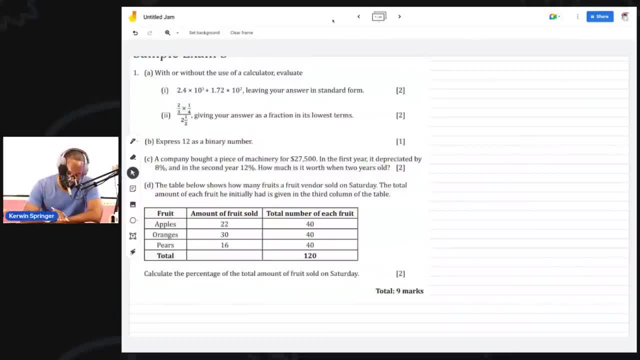 A company bought a piece of machinery for 27,500.. The first year it depreciated by 8%, it was, and the second year by 12%. How much does it do it when it's two years old? So after the first year, how much is it worth in terms of a percent? 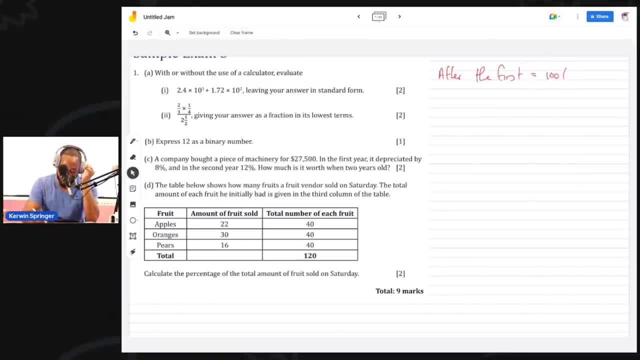 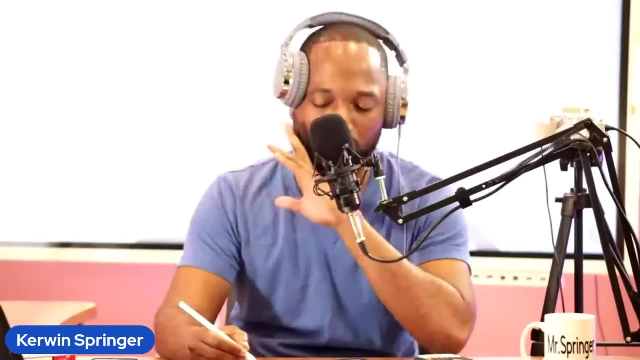 It is equal to 100% of the value minus the 8% it depreciated. So this is 92%. So, and after the second year we need to get 12% less. So there's a way you can do it shortcut with percentages, but let's not go through all of that. 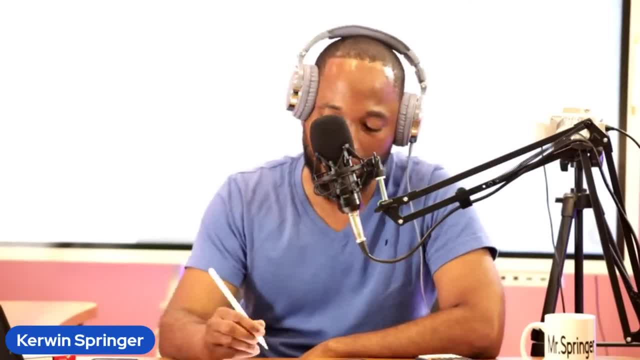 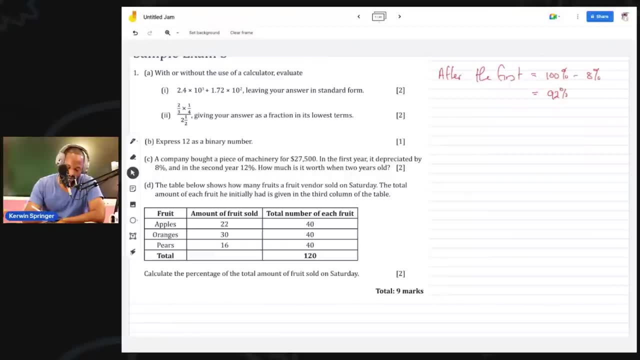 I could just do 0.12 and wait out of the 92% and that kind of thing, But let's keep it in the general way that everybody would approach this question. So once again after the first year, in terms of money, yeah, 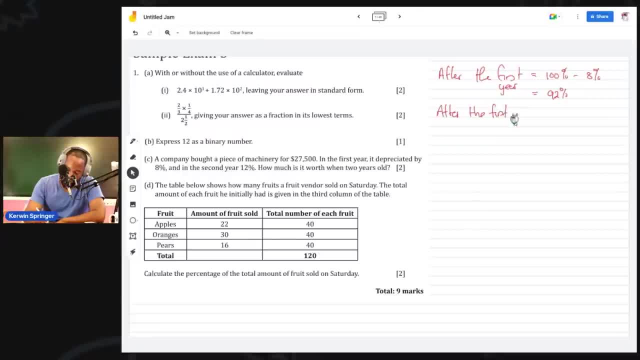 After the first year. in terms of money, we expect 92%, which could be written as 0.92, multiplied by the 27,500.. How much is that? That is 25300.. Making sense? Yeah, that's sounding like a fair number. 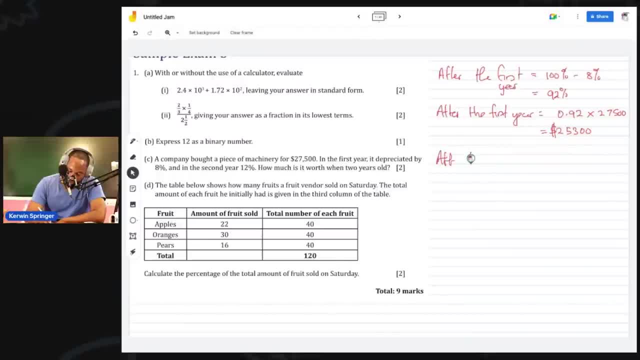 So after the second year It's going to be equal to 100 minus. it's going down by 12% in the second year. What is going on with this machinery? 12%, So it's now 88% of first year value. 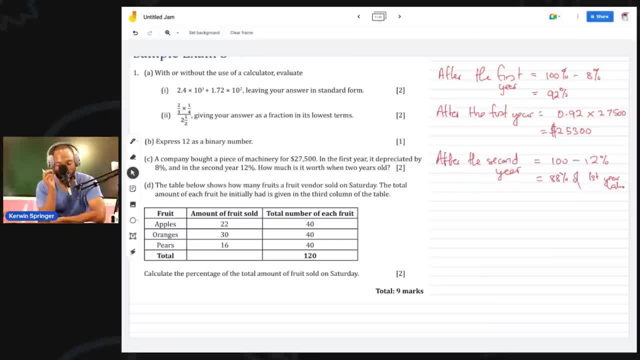 Not the zero years Now, when you buy it initially after the first year, So after the second year. So it is worth It's 88%, which is 0.88, or 88 over 100, multiplied by 25300, which is 22264 after the second year. 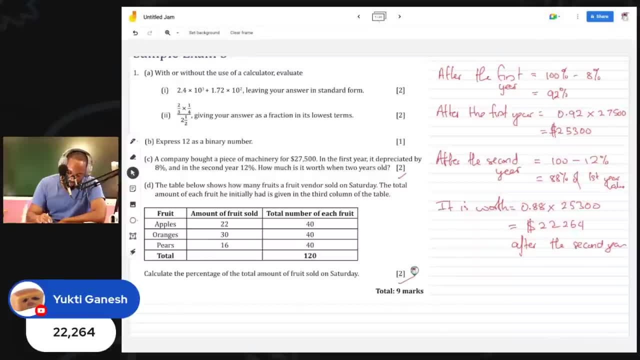 And you get two marks for that. So let's go ahead and get our last two marks here. What is going on Table below Shows how many fruits a fruit vendor sold on Saturday. The total amount of each fruit he initially had is given in the third column of the table. 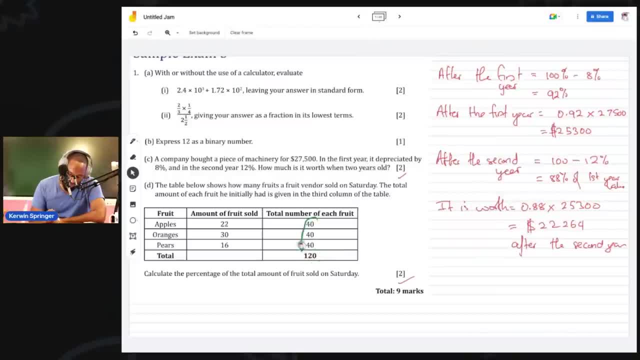 This is the amount of fruit he had initially And this is the amount of fruits he sold. Calculate the percentage of the total amount of fruits sold on Saturday. What kind of standard for question is this one? Let me make sure I lost the marker. 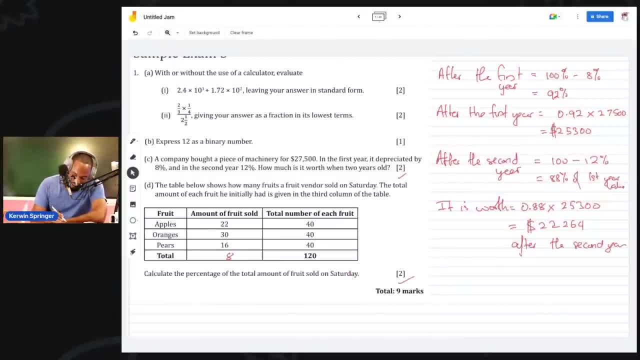 So this is an eight And this is a how much Right? 58 fruits. he sold No, 68.. 68 fruits sold. So if he sold 68 fruits And part D, If he sold 68 fruits, The percentage sold: 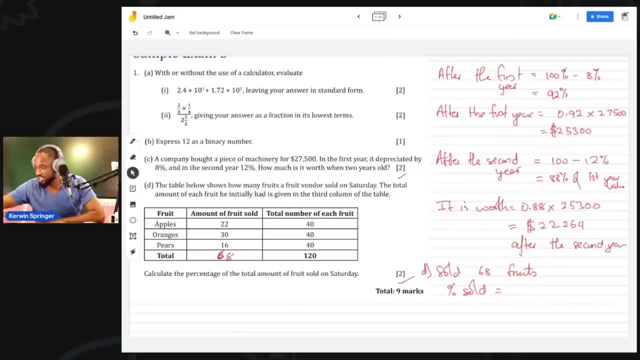 Would have to be So- nobody put your hands on the chart yet- Would have to be 68 out of the 120.. Multiply 100 over one And what your calculator telling you? that is 56 and two-thirds percent. 56 and two-thirds percent. 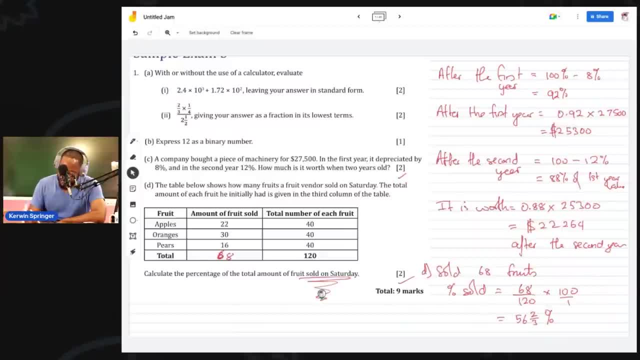 Now they didn't sit around it after anything, So I'm keeping the exact value. So I'm keeping the exact value If you're wrong. It shouldn't be 56.6.. It should be 56.7 or 56.67 or something like that. 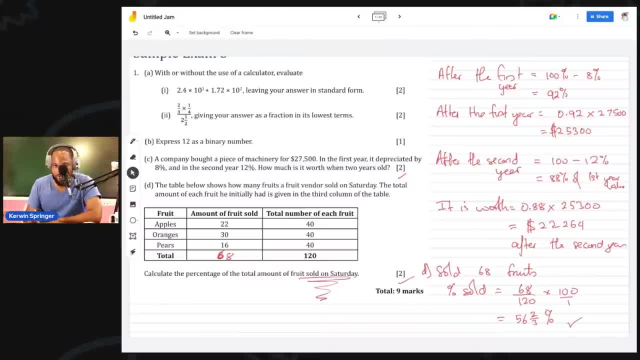 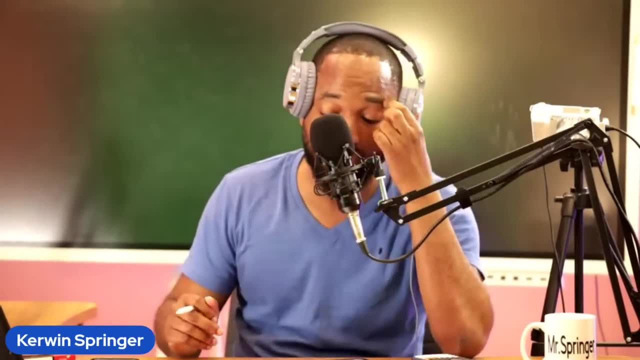 But I'm keeping the exact value, 56 and two-thirds percent, And that's it. These question ones. You feel you're going to crack me full. nine marks in question one. You're ready for anything. Are we taking the next one? 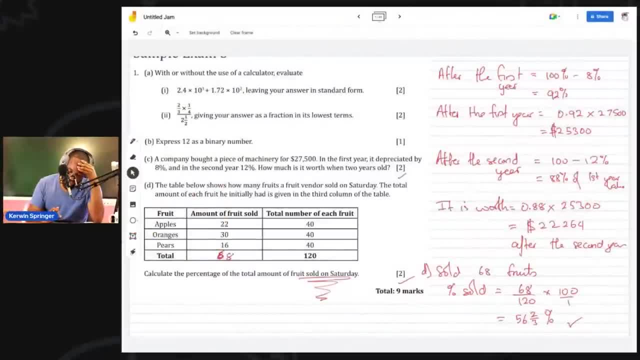 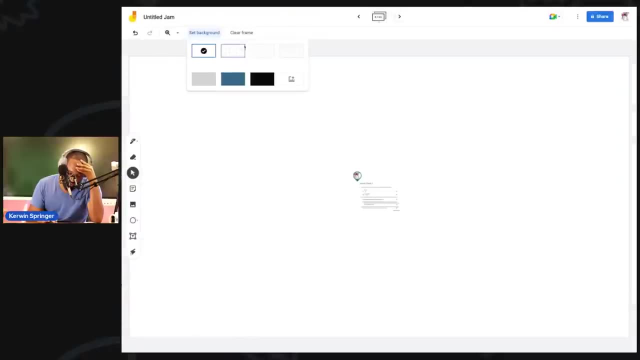 It's starting to get fun now by you. Usually in studying it have a few stages that you would pass. There you go, so you start studying. the hardest thing to do in studying is to start, but initially, after you finish one or two questions, you may feel to stop. 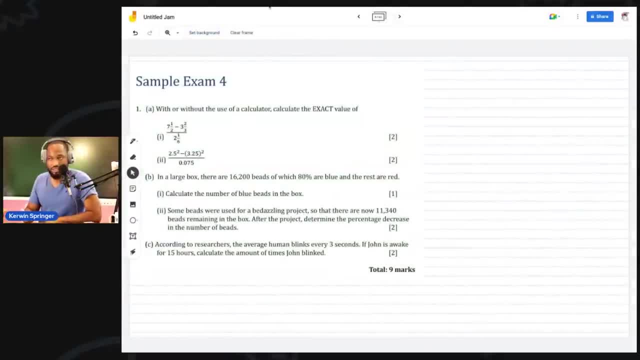 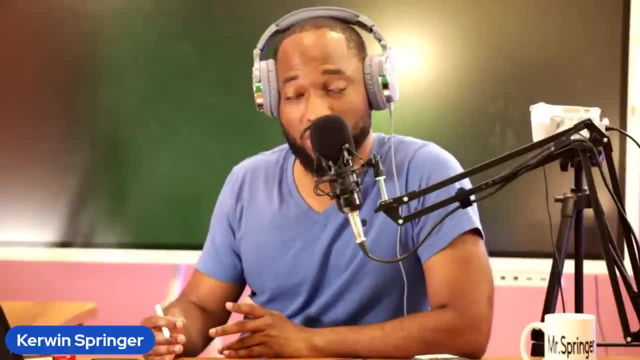 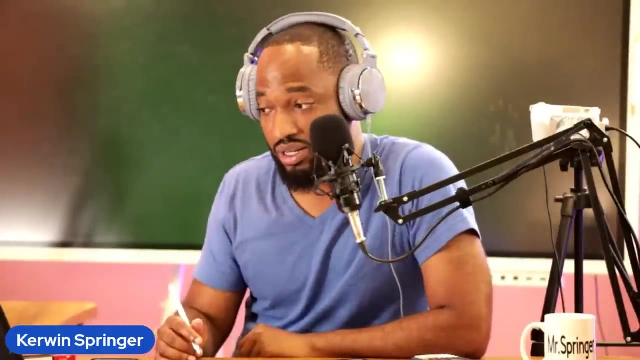 but then, if you keep pressing, there comes a time where you get in the zone and, boom shot, you do a two hours, you do a three hours, you surprise yourself four hours of studying straight. and it was productive. it was learning things for real. so lean into that right now. 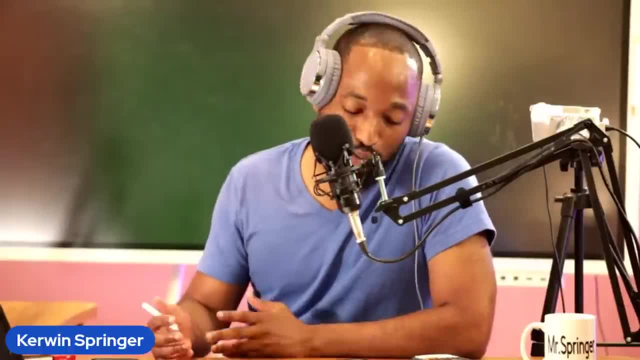 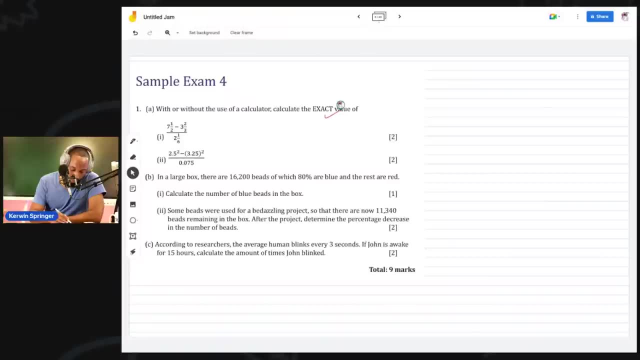 there's no more time. there's no more time to procrastinate. give yourself a fighting chance. so, without the use of a calculator, calculate the exact value of boom and bang. so let's see if you could just ramble up that real fast. this is exam four. 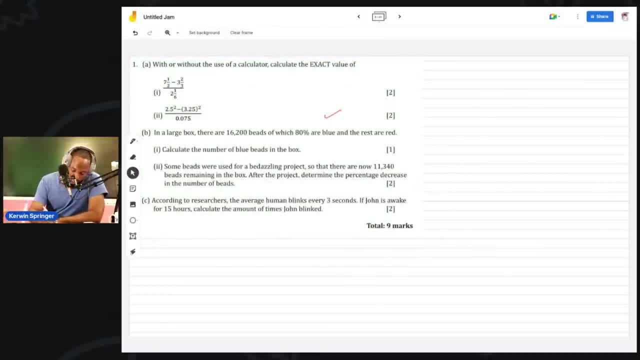 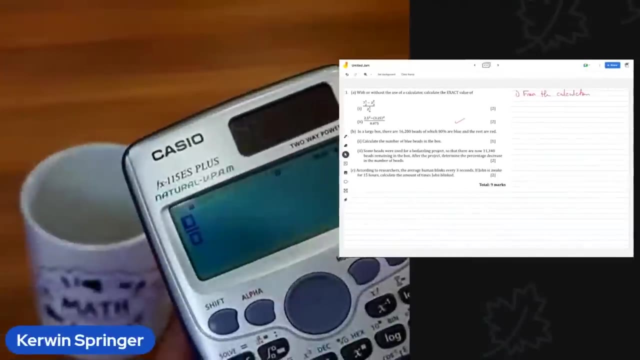 from the calculator for the first part. what are we getting? exact value. so it would be back to using fractions. exact value means keep it in the fractions. so what I'm gonna do, I have the fraction set, I'm gonna press shift and the fraction to get that mix number vibe. 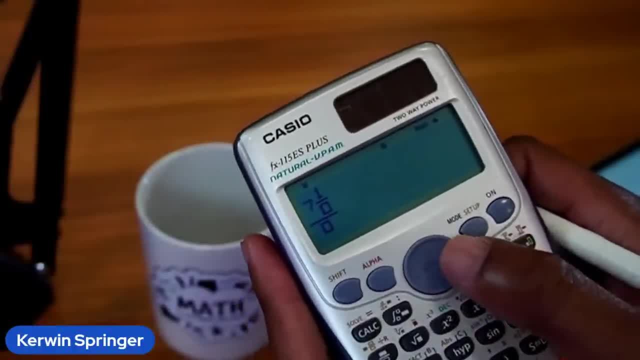 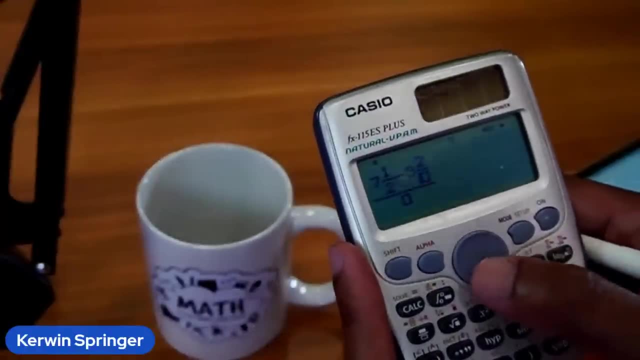 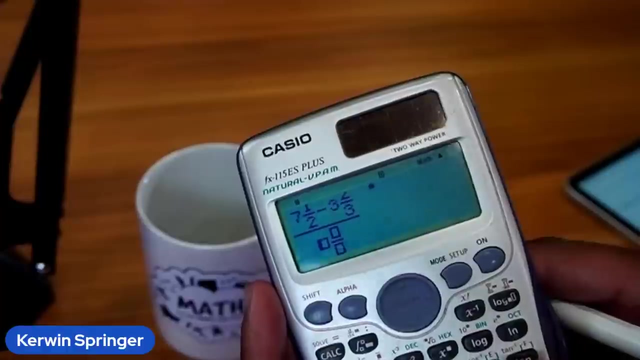 seven and a half. it's important, it's imperative that you learn how to use your calculator for this. that's the skill they test in here: three and two thirds and shift again and that and I'm putting. I know there's a little glare so I'm kind of just splashing it across so you can see. 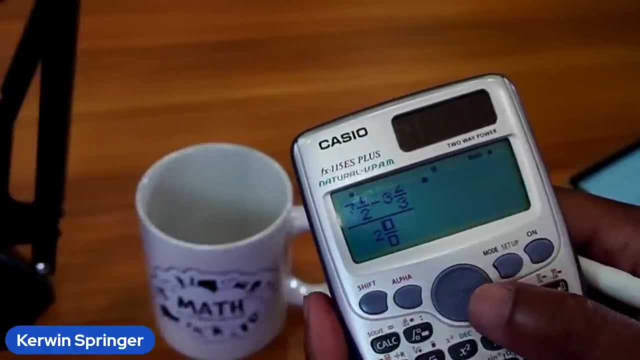 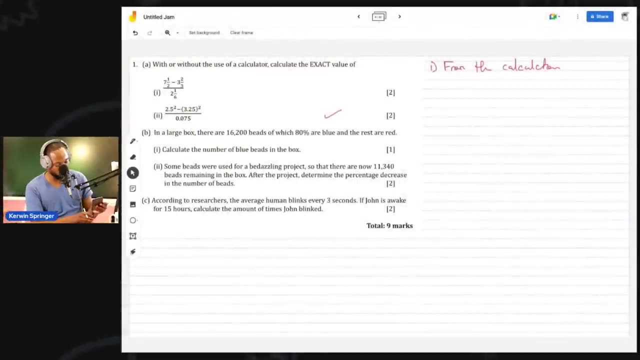 two and one sixth, twenty twenty three over thirteen. I don't see no answers there. I don't see no answers there, so for part one, I'll put the answer as soon as I start doing the question, as soon as I see the question, so from the calculator. 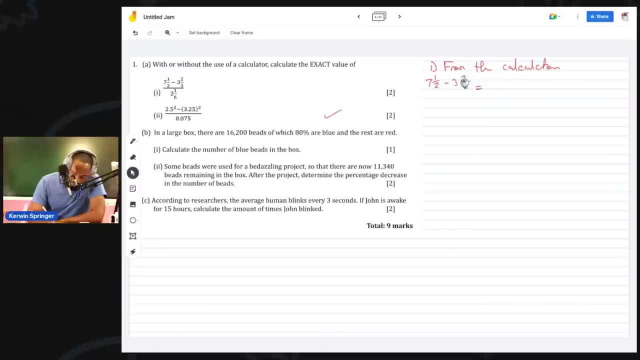 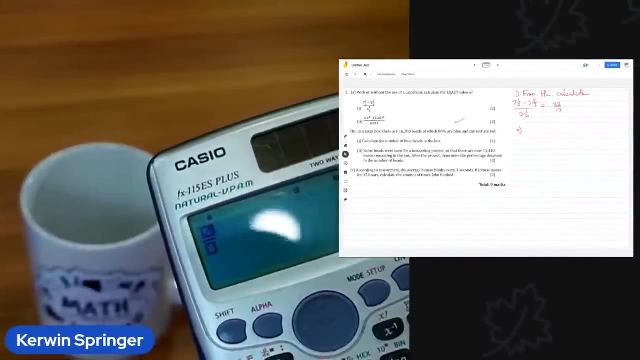 all of this is equal to twenty three over thirteen. and for part two, calculator time again. come on, boy. so I don't know what was that 2.5 to b squared. so like to test the use of indices if you really know how to do the thing for real, for real. 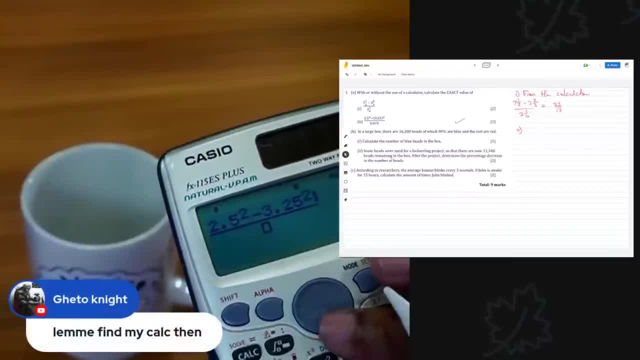 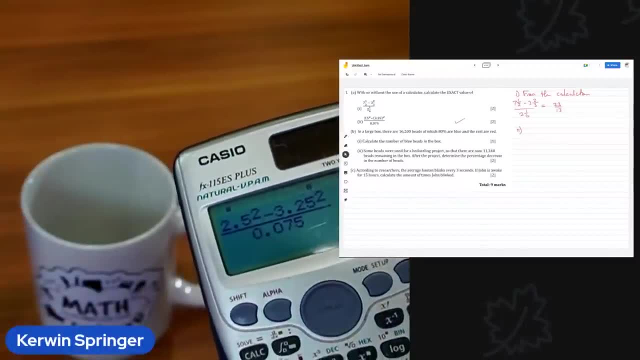 3.25 to b squared. you can put it in brackets, but I know my calculator. I know my calculator. how am I back there? 0.075, 0.075, 0.075. let's check a negative number now. it's very rare that I get a negative number. 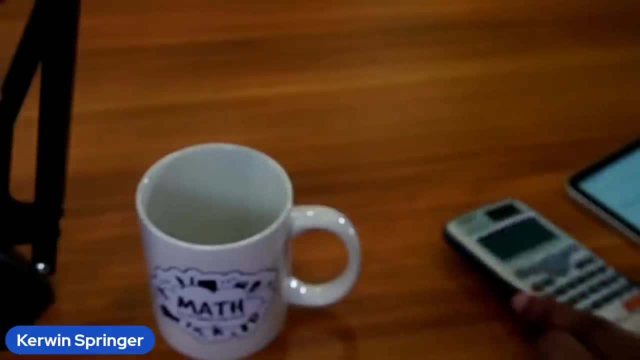 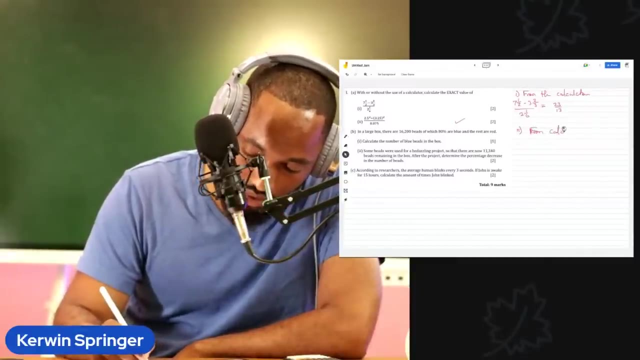 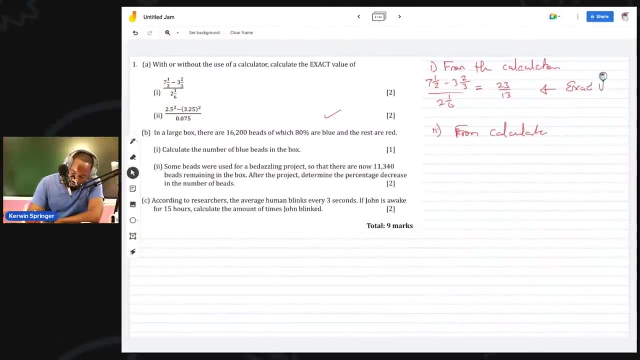 in this case. so they usually do test, they'll bring up the negative numbers here. so this is 2.5 from the calculator. by the way, this is the exact value for the first one, so I'm not going to change it. the exact value from the calculator. 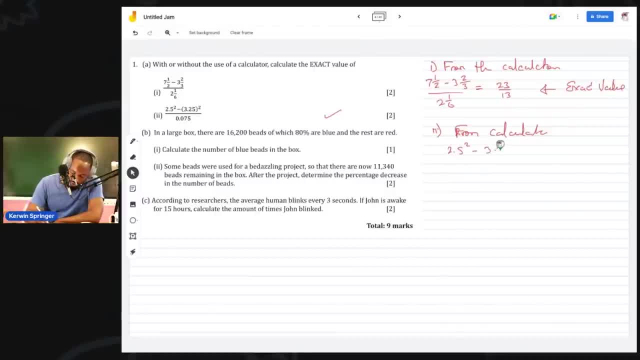 2.5 squared minus 3.25 squared over 0.02. zero seven five is equal to negative one. one five over two. brilliance part b: in a large box there are sixteen thousand two hundred beads, of which eighty percent are blue and the rest are right calculated. 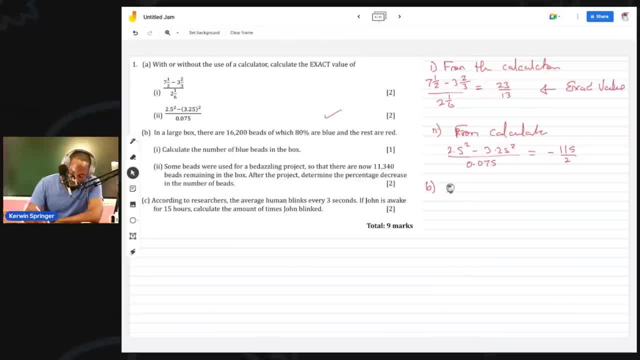 that question too easy, but let me skip that one. so blue beads is going to be 80 percent, which is 0.80, multiplied by 16, 200, which is one, two. yeah, well done, i hack one, two, nine, six, zero blue beads. and for part two, some beads were used for bedazzling, for a bedazzling project. 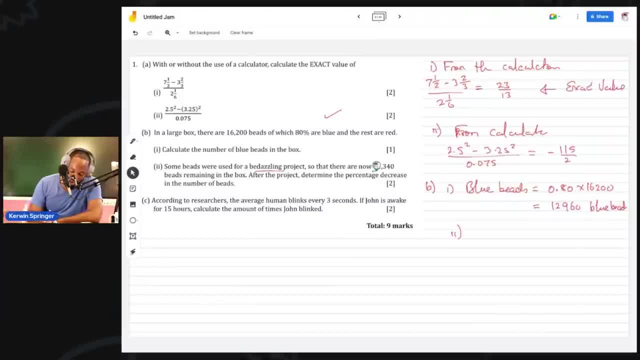 so that there are now eleven thousand three hundred and forty beads remaining in the box after the project determined the percentage decreasing the number of beats. so, uh, they just tell you about our direct beads for kick. so i find that could be part of the question too. anyhow, so it did decrease. 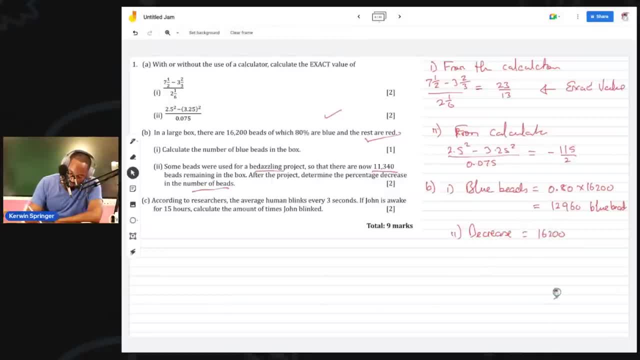 is one, six, two, zero, zero minus one, one, three, four, and then you take that number and put it over the original and multiply by 100 over one to find the percentage decrease. so the percentage decrease is whatever that number was. so i could put it back: one, six, two, zero, zero minus one, one, three. 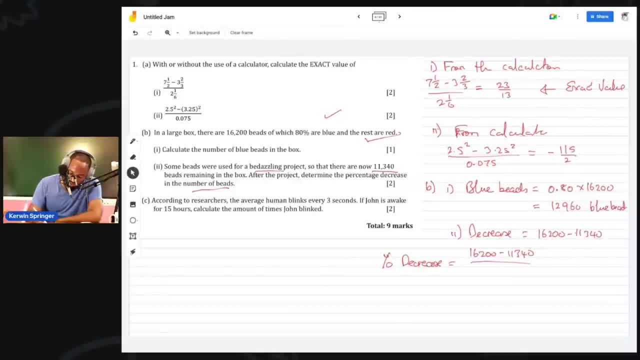 four zero. i could write the number over the original, multiply by 100 over one, and for that you should get 30 percent. can i get to the percent i'm i'm feeling at 30 percent? according to researchers, the average human blinks every three seconds. 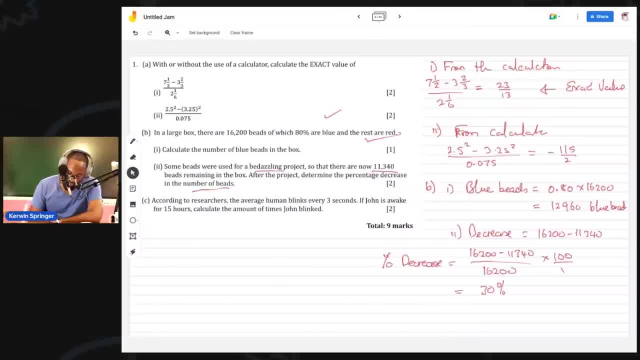 so if john is awake for 15 hours, calculate the amount of time john blink. so every three seconds you blink. my right now research that that was that that was not true. that was not true. three seconds, one, two, three blink. nobody you blink like that if, if your exams are on the corner. 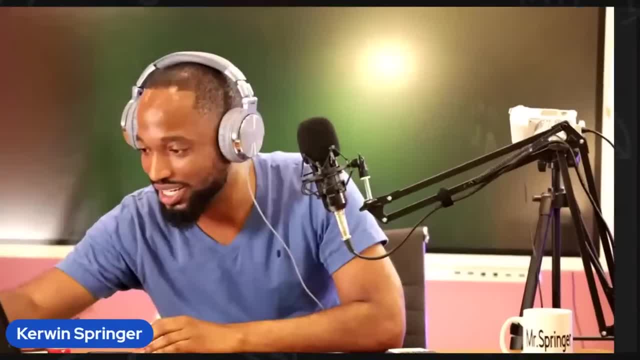 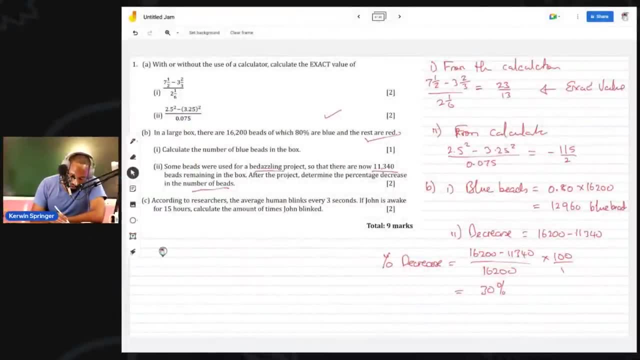 maybe that maybe, if your exams are on the corner, you're breaking like that. all right. so according to researchers, the average human blinks every three, three seconds of january, 15 hours. so we just need to find out how much, how much seconds in 15 hours. so in one hour there's 16 minutes, so it's 15 times. 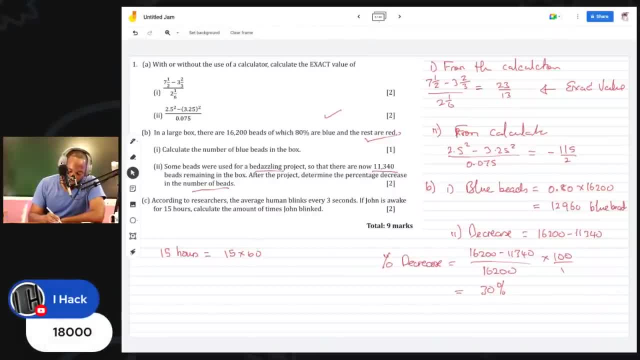 60 in minutes now, and in one minute there are 60 seconds. so it's 60 times 60, or 60 times 63, 600, and when we multiply that we get five, four, zero, zero, zero seconds, and you blink in every three seconds. so 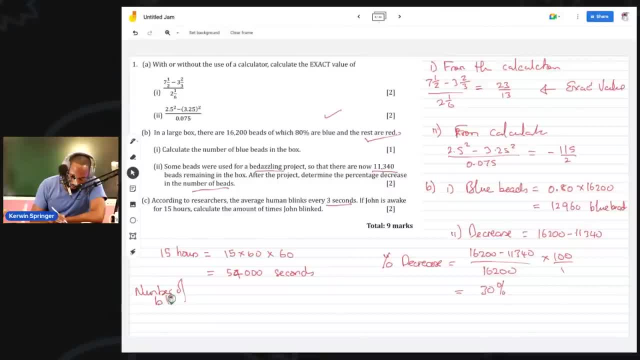 number of blinks is going to be equal to 5 4 0 0, 0 divided by 3, which is, according to the chat, 18 000 is correct, just like that. we rack up our next question when i do one more. one more for the road, one more for the room. 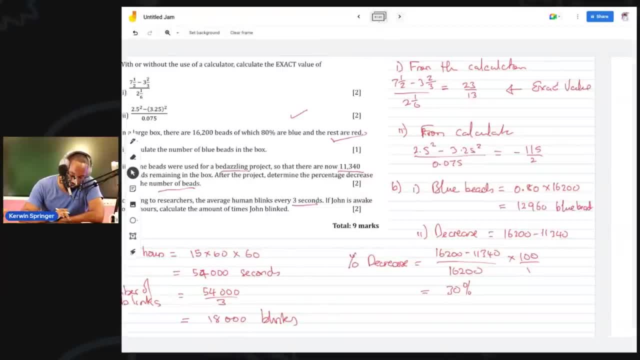 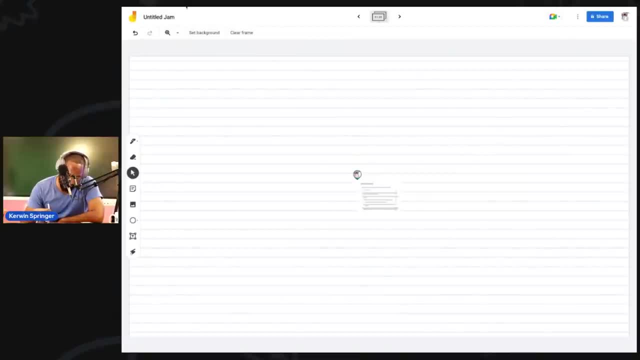 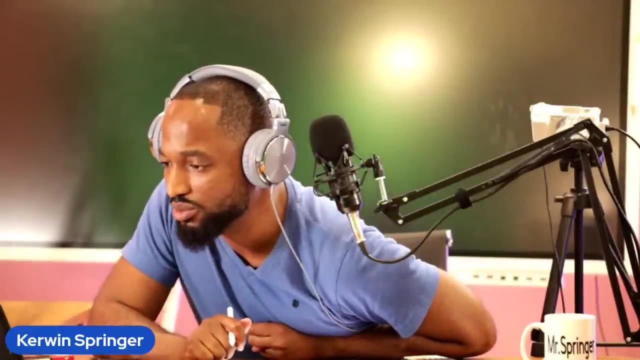 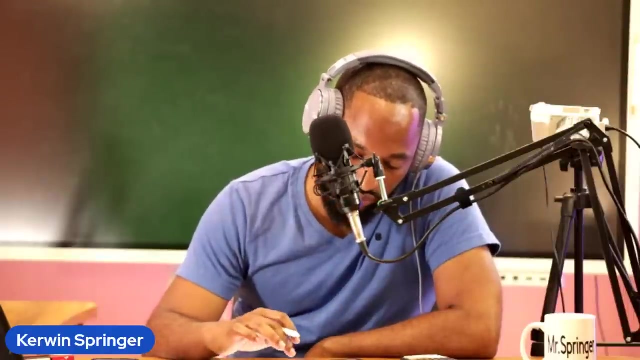 one more for the road. how much is this? we do, right, five, yeah, i think we do five. five quick, quick, quick. and how long we live? 46 minutes, not bad, not bad. tomorrow we try and do five algebra questions. wait. so, without the use of a calculator, calculate the exact value of. 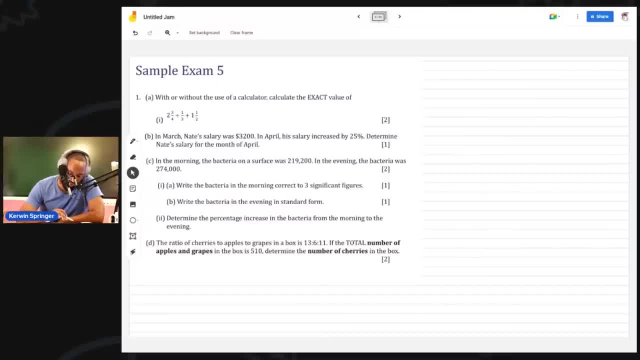 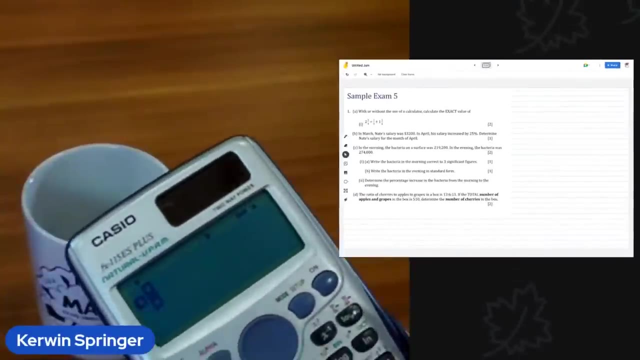 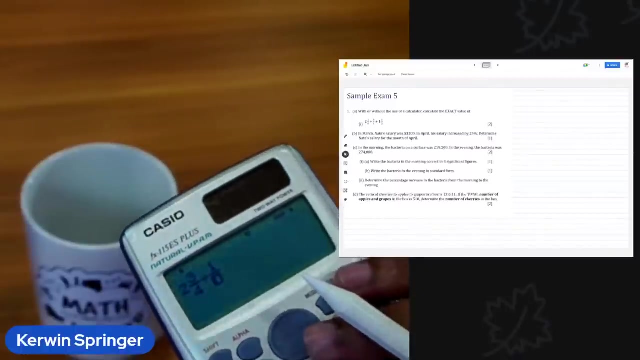 two and three quarter divided by one third plus one and a half. i'm fed up at this boy. all right, all right. this is invigorating me. i can do a million of this. i love this. two and three quarter, uh, divided by one third plus one and a half. 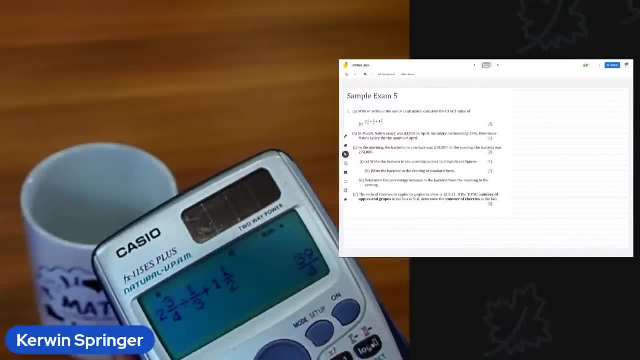 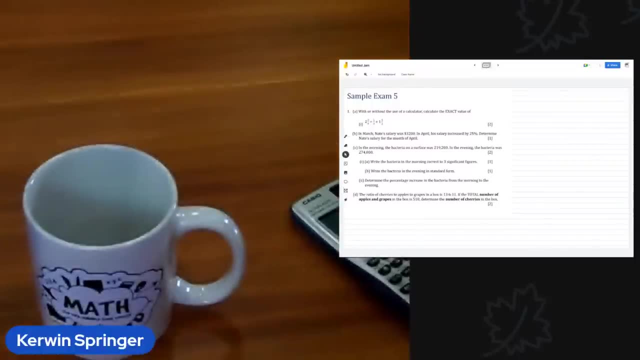 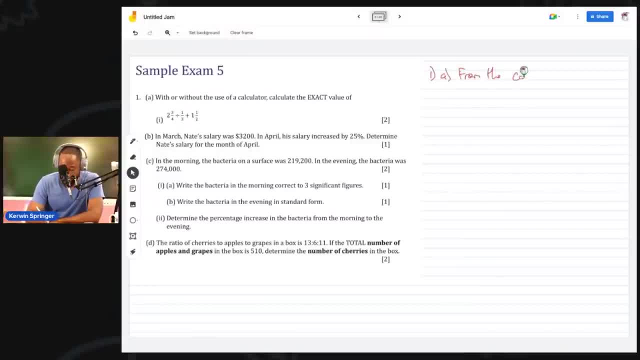 from the calculator, the best calculator we have- that two and three quarter divided by one and a third plus one and a half is equal to 39 over four. that's the exact value. part b: in March need salary was this amount. In April, salary increased by 25%. 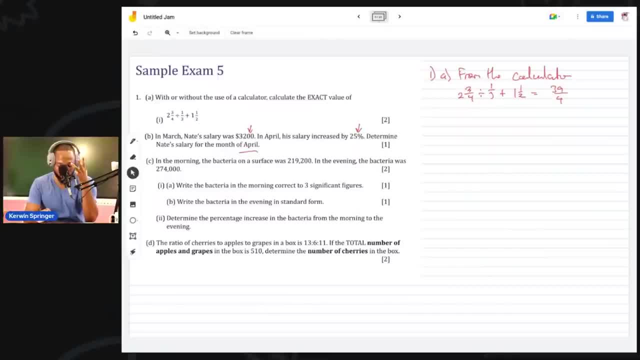 So they bring in percentage increase in three ways and we didn't get to see the hard way. I'm sad that we didn't get to see the hard way. There's a way that they can bring it where they give you the final value. 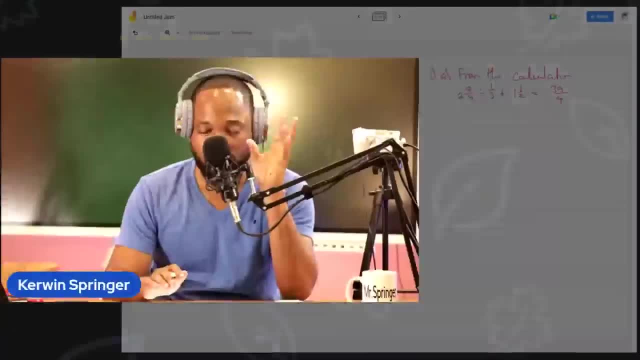 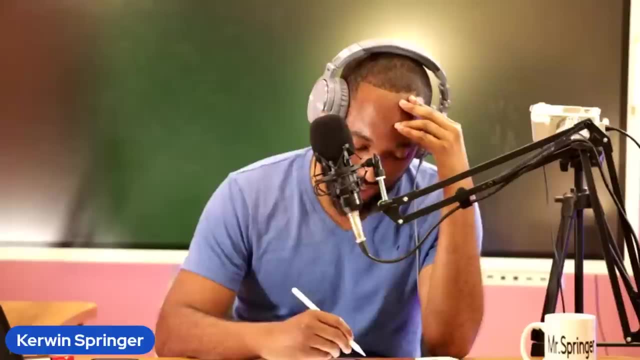 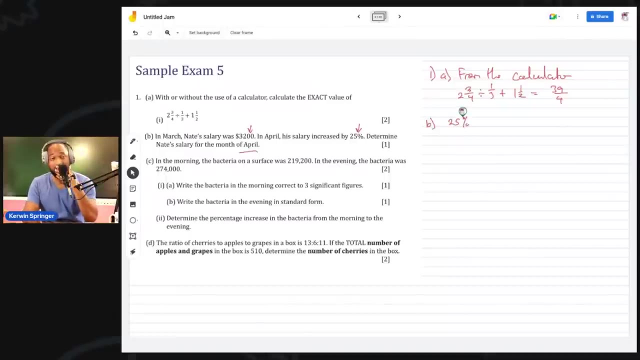 and the percentage increase And there's a little thing you have to do. You have to equate the percentages. But in this this is easy. How much percentage increase? For part B? it's a 25% increase. My weekend was so good I had a bus slip. 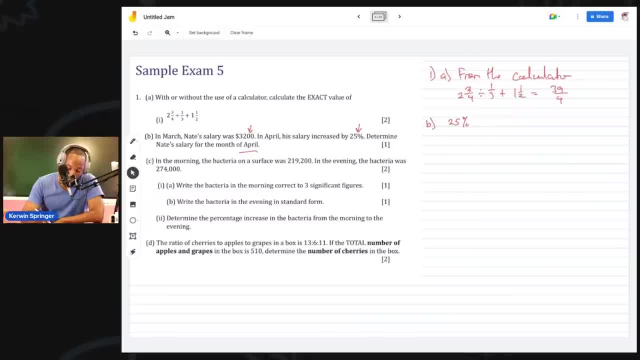 You know your weekend is good if you come in Monday with a bus, slip 25%, But I wasn't fighting in the airport or anything. 25% increase means 125% final value. So new salary Taking way too long for this one Mark. 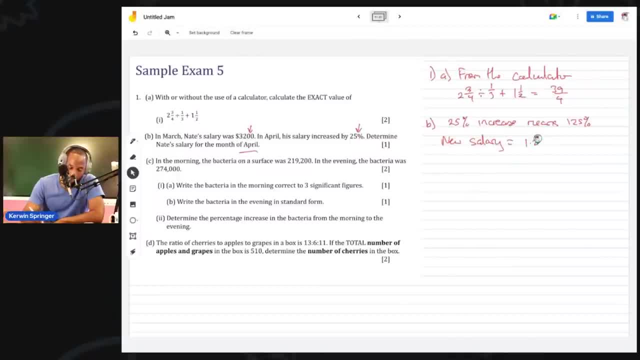 New salary is equal to 125%, which is 1.25.. 125, 100, multiplied by 3200, which is 4,000.. 4,000.. All right, so let me do this one. In the morning, the bacteria on the surface was this amount: 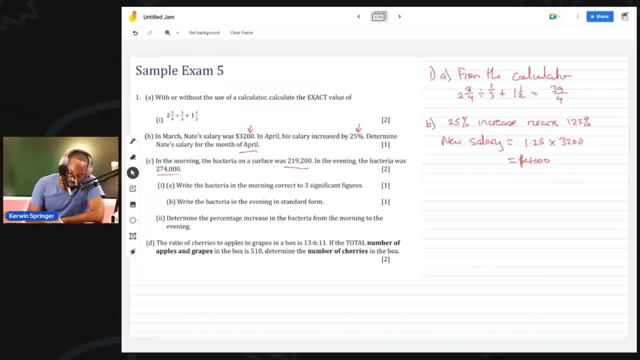 In the evening it reached that amount of bacteria, going up by The bacteria in the morning. Wait, wait, wait. How is that? two marks here? I'm not supposed to be there. One, two, three, four, five, six, seven. 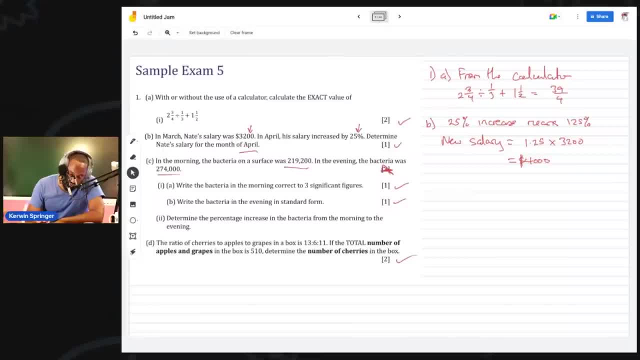 Something's suss about this question, Sussness Right. the bacteria in the morning corrected three significant figures. So in the morning corrected three significant figures is 219, and they changed all the rest to zeros. Two, three significant. 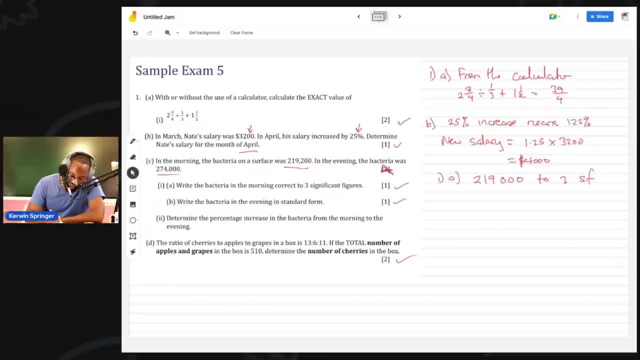 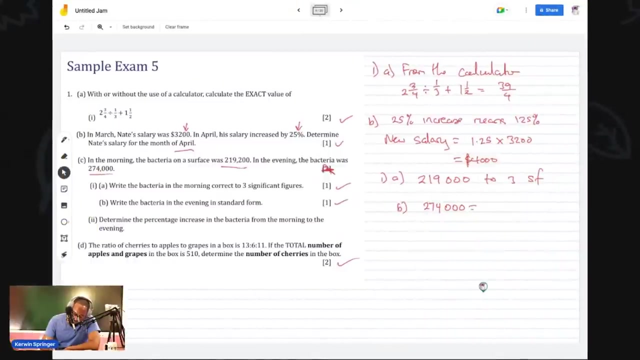 Two, three significant figures. The most significant figures are furthest away. The higher place value, the more significant. All right, the bacteria in the evening in standard form. So it's 274, 00, zero. In standard form, that's 2.74.. 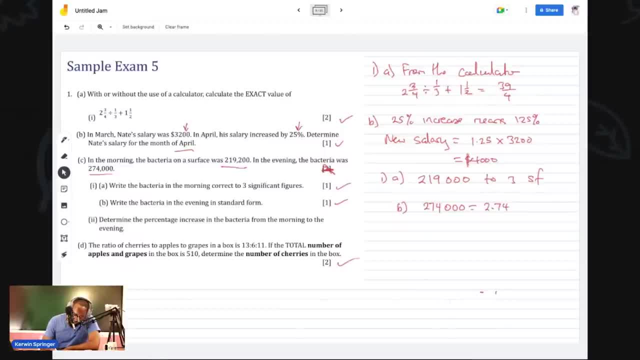 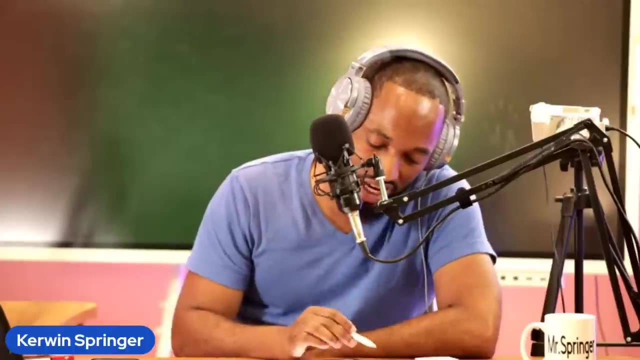 And how many times you move the decimal point One, two, Three, four, five Times 10 to the power of five. Y'all got those two answers. Yeah, why'd you show them, Mike? Now a lot of y'all in the chat. y'all just put 219. 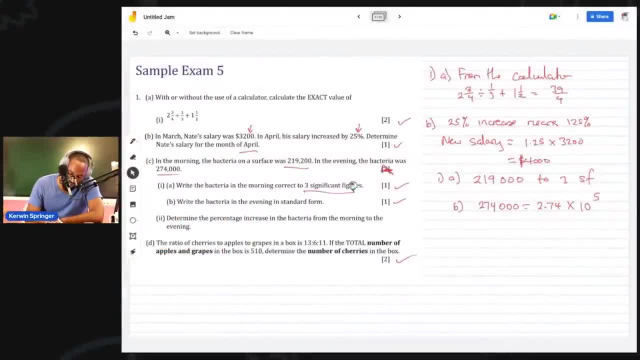 A lot of people just do that for significant figures. They just write this and then forget to write back the zeros. If you put 219, then you get wrong enough. And the percentage increase. Oh, there's the two marks here. Two marks here. 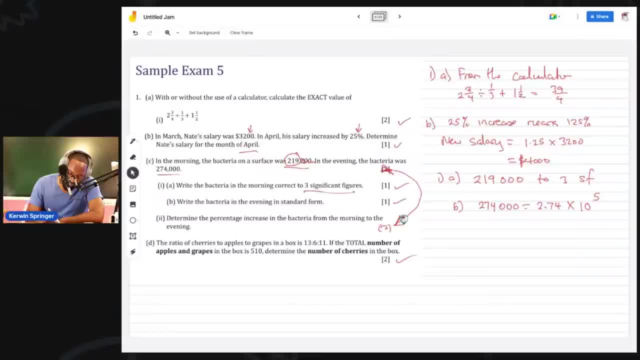 The percentage increase in the bacteria from morning to evening. So the percentage increase we do this just now is going to be 274, 00, minus 219, 00, over the original 219 is 2, 2, 00, 219, 2, 00, multiplied by 100 over 1.. 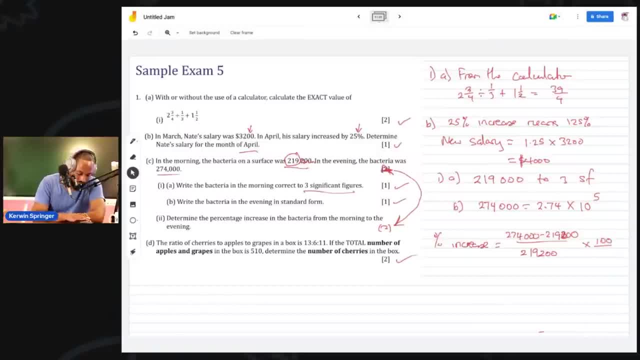 How much y'all get with that? 274, 00, minus 219, 2, 0, 0.. Well, we're finishing this life in a short time: 219, 2, 0, 0.. 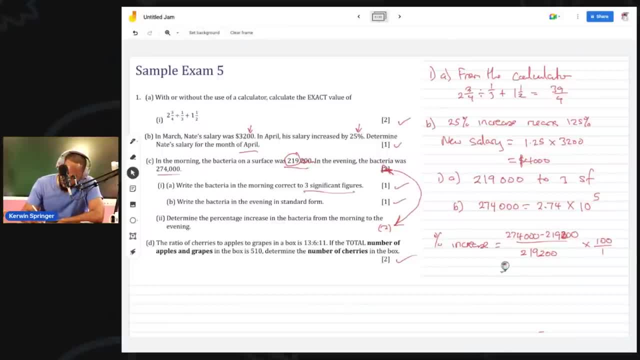 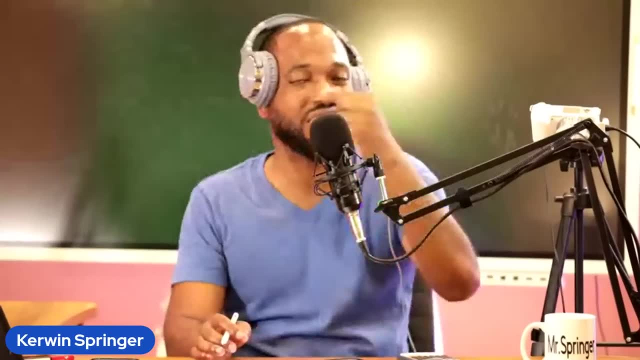 A quarter of 100.. I'll get 25%. So this is 25%, boy, And the last one the ratio. So we get a lot of ratio questions here And CXU. I love ratios these last few years. Chances of a ratio question. 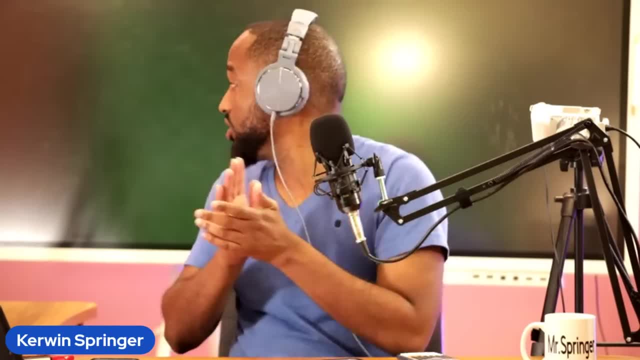 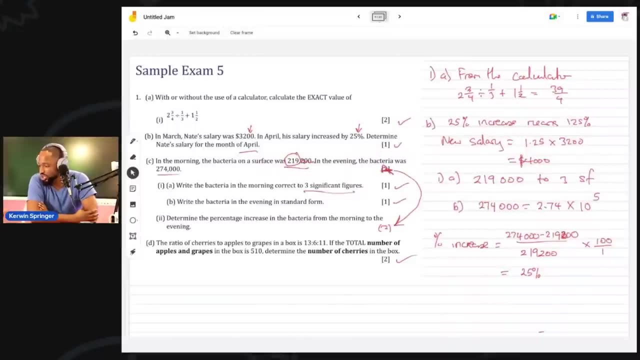 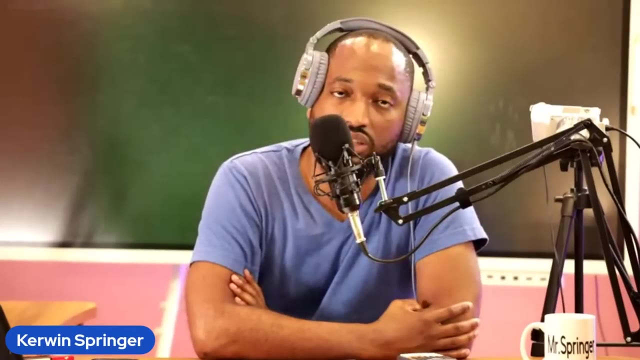 Hey, 319 people here. Congratulations for being here and studying with me. Yep, See, good to see you. Which country you're from? Shout out your country. Chances of you getting a ratio question for the exam is pretty high. 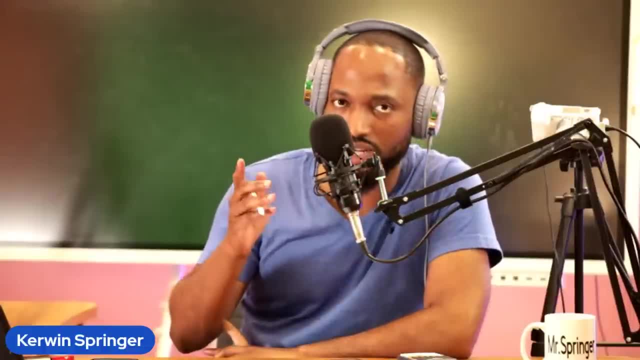 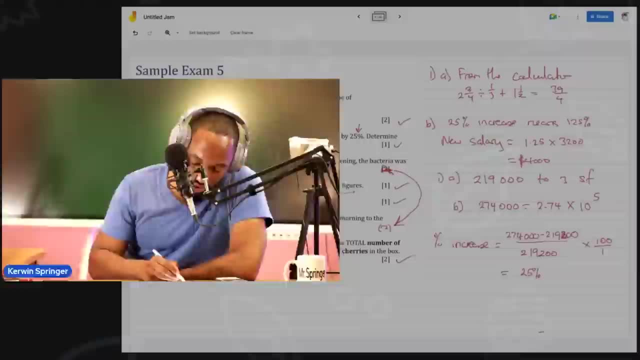 So make sure you know how to do ratios, even the weird way, how they bring it Where they don't give you. It's hard to figure out for one year the subtract two of the parts, If the total number of apples and grapes in the 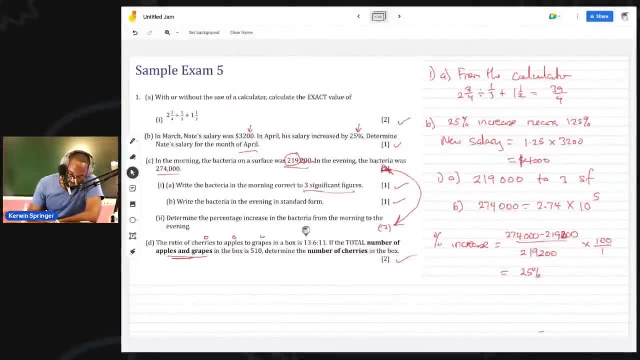 This is the ratio of cherries the apples the grapes, Cherries the apples the grapes. If you do, the number of apples and grapes is 5, 10, it's too many number of cherries. So the key for ratios question is finding for one. 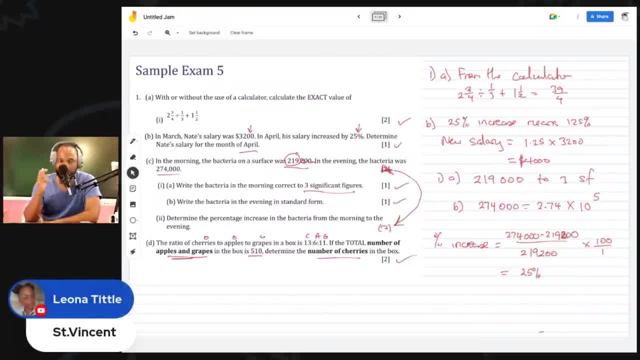 You need to find something to equate the parts, the number, and then find for one part. So apples and grapes represent how many parts. Six plus 11 equals seven, Yes, Fifty. 17 into four or three, seven, yeah, seven, 30,, 30..